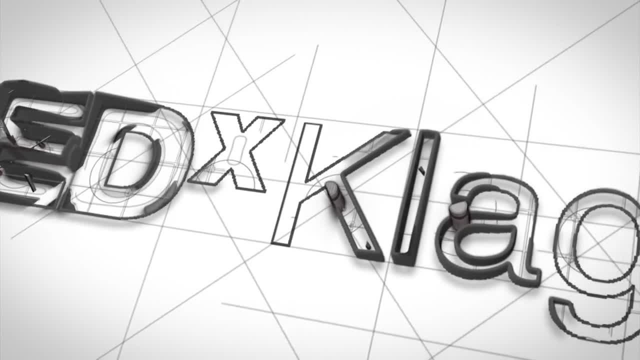 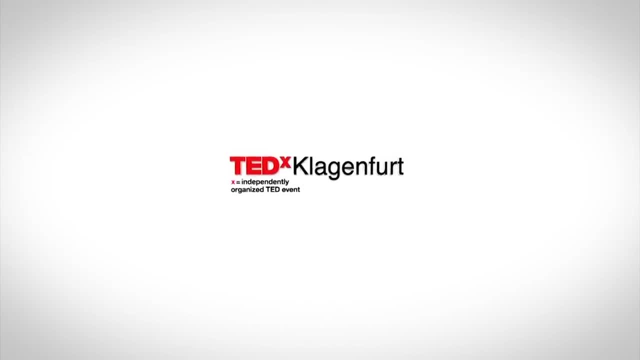 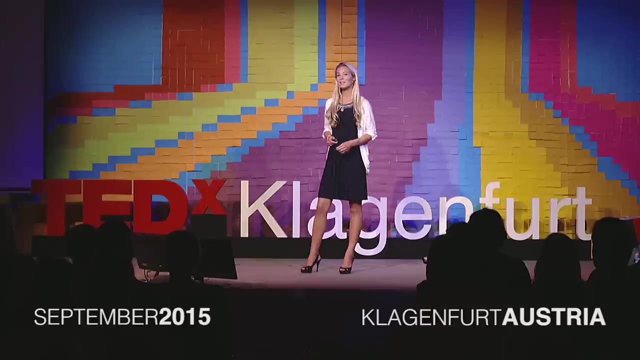 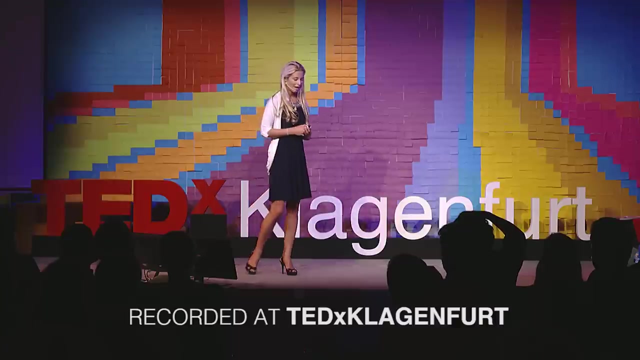 What if we were to redefine the relationship we have with sharks to one based off scientific fact, reality and logic, rather than the current one, based off of limited and biased information? I want to talk about how changing the way we perceive sharks and interact with them could change our environment, economies and 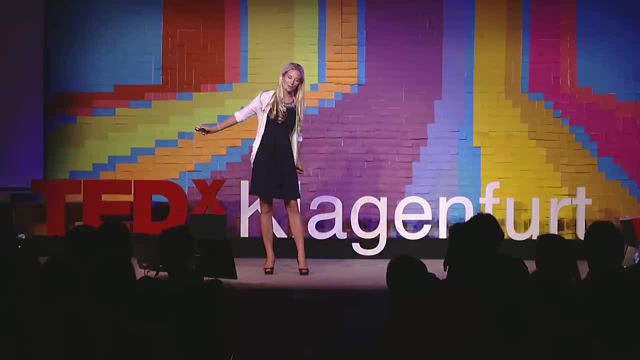 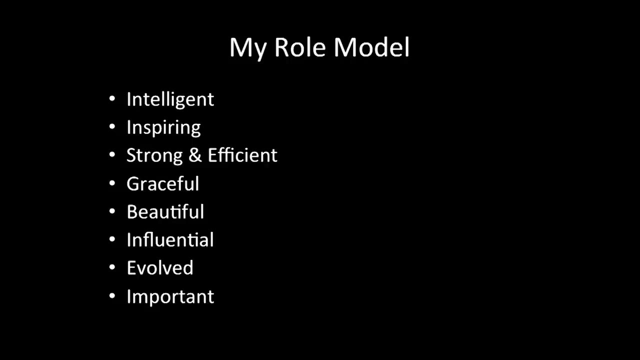 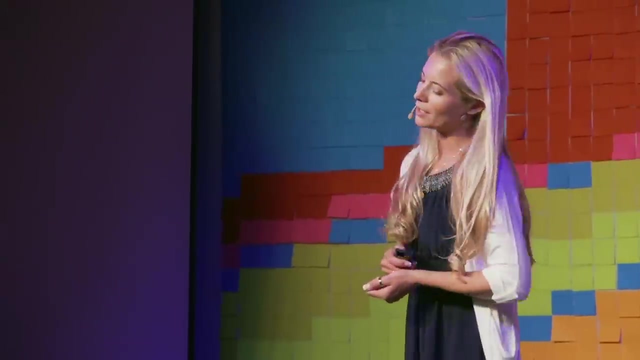 lives for the better. But first I want to introduce you to someone who has positively influenced and inspired my life's work, passion and focus. She's intelligent, she's graceful, beautiful, efficient. but what I admire her most for is her very important. 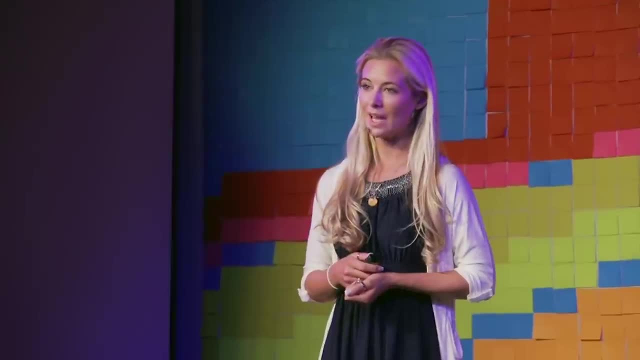 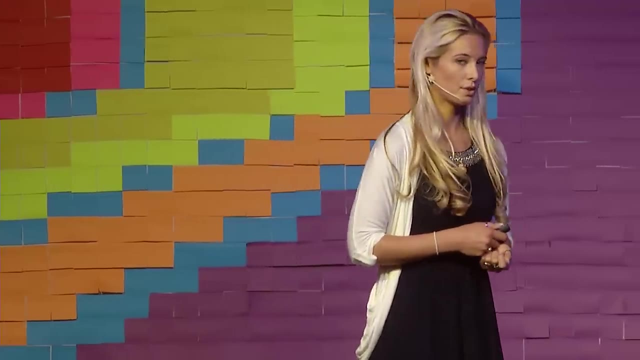 work and role. And what most people don't know is that without her work and influence, none of our lives would be the same. And I wanted to describe her to you first, before I showed you her photo, because I've come to find that oftentimes we make snap judgments. 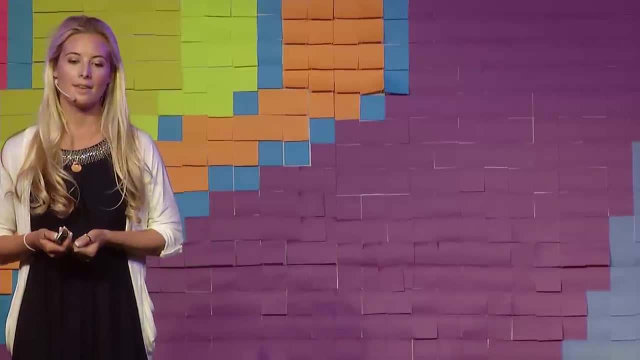 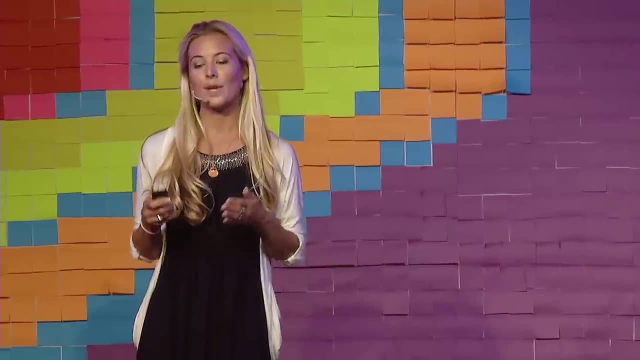 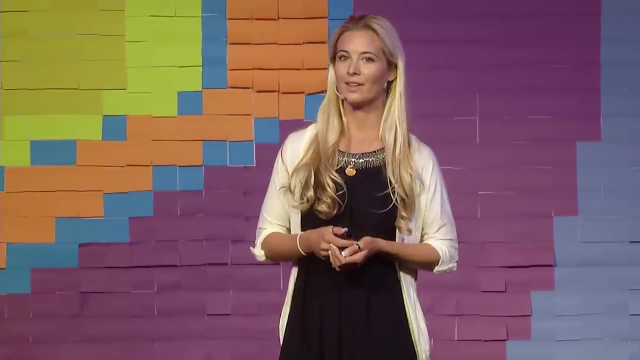 prejudice based off of very little factual information, And I've personally found this because oftentimes I'm judged solely off of my appearance or work as a professional model, rather than my primary work in science, conservation and business. So please keep in mind the truth. 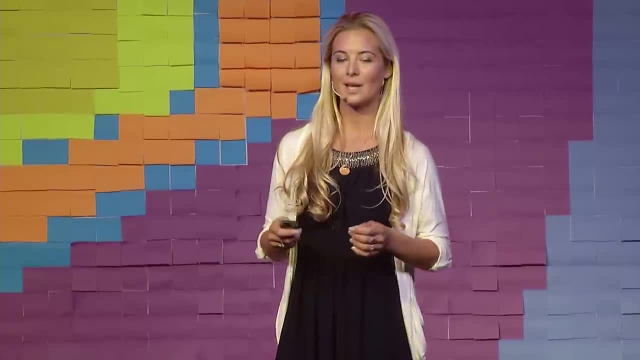 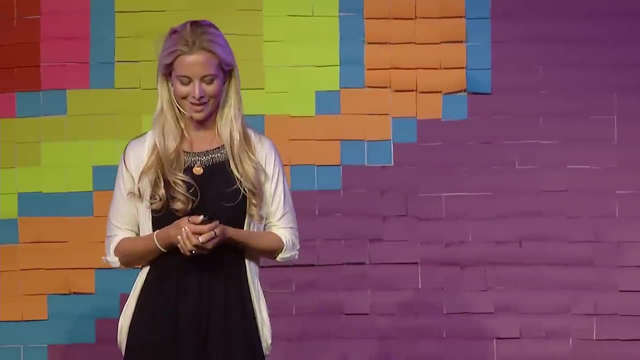 that often there's more than meets the eye, and when you take time to get to know someone and better understand them, maybe you can better value them, And sometimes it's a little bit more interesting than you think too. So, without further ado, my beautiful role. 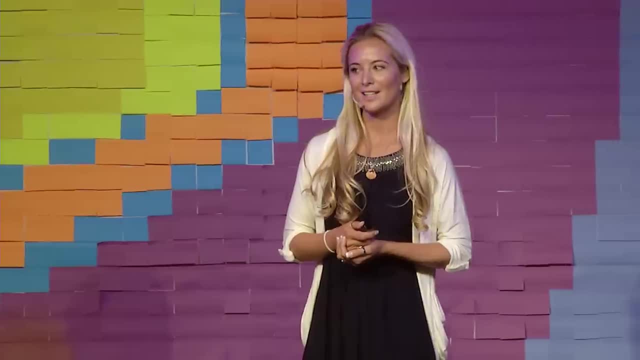 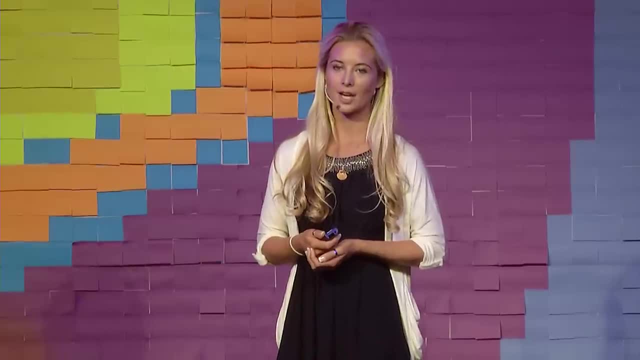 Bella. And yes, this is my beautiful role model, Bella. And yes, this is my beautiful role model, Bella. And yes, she's a great white shark, or more accurately termed a white shark Carcaradong carcarus. now I know you might just be noticing her nice teeth, thinking something. 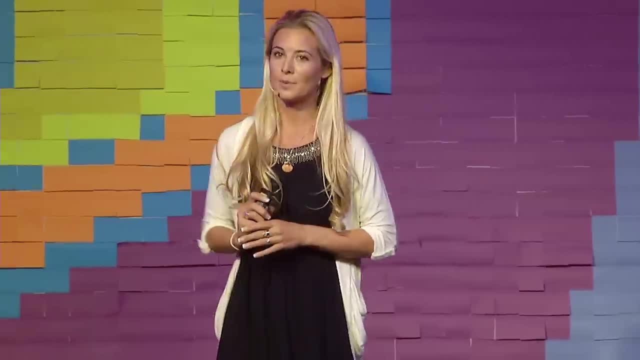 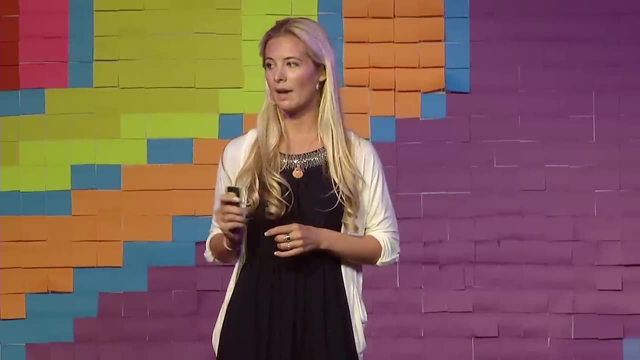 along the lines of monster. But tonight I want you to put your prior beliefs about sharks on hold. I will explain why Bella is actually such an ideal role model and why we should seriously take action to redefine the relationship we have with these animals to one based off. 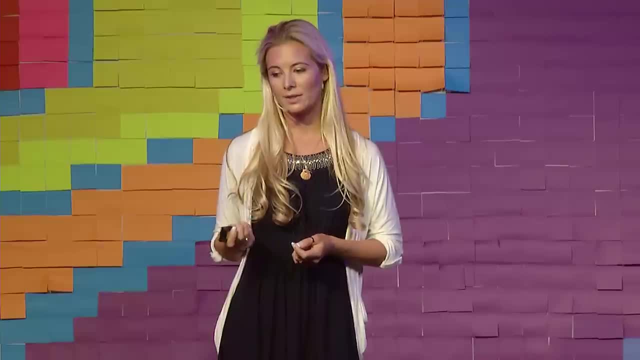 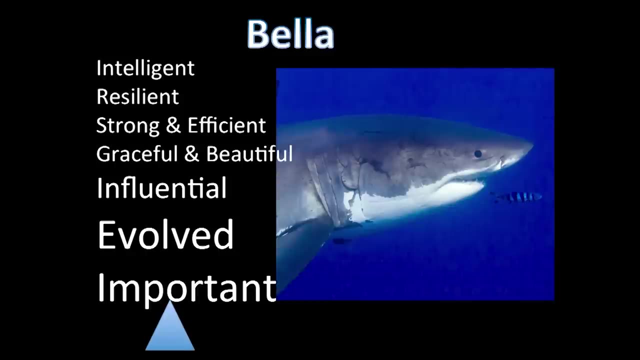 scientific fact, data, reality, rather than appearances, snap judgments and fictitious Hollywood movies. so Bella and her kind are extremely intelligent. I've observed her and her kind outsmarting even humans within a matter of moments by adapting her behavior, even in novel situations. 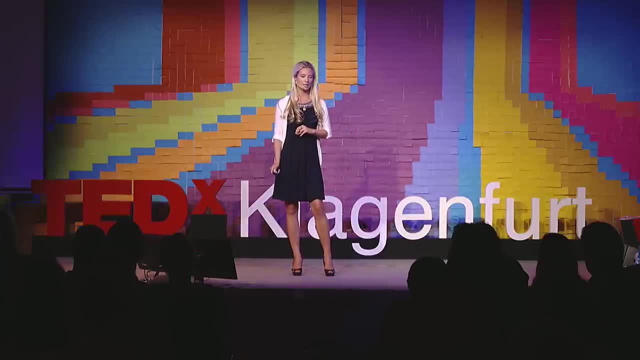 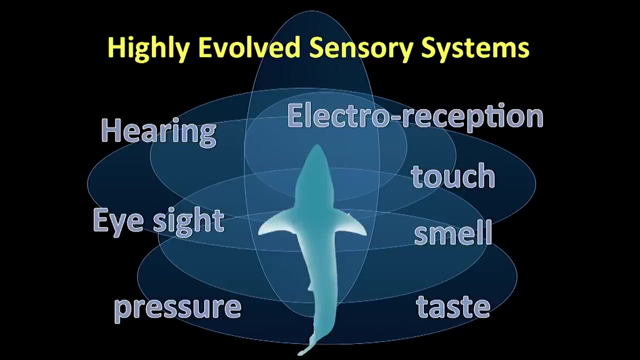 This ability to quickly adapt has likely led to sharks' resilience over time. They evolved before dinosaurs, before trees, and they evolved two more known sensory systems than we even have to give them a high level of efficiency in their very important role in ecosystems. 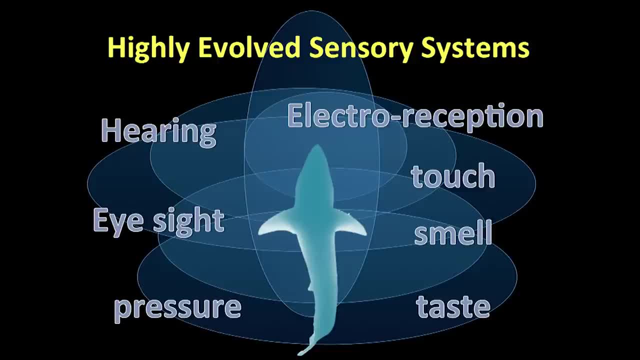 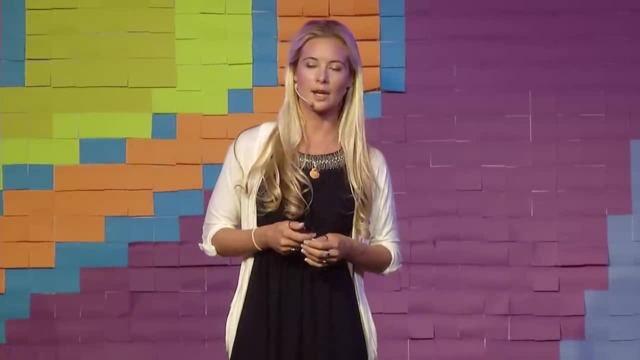 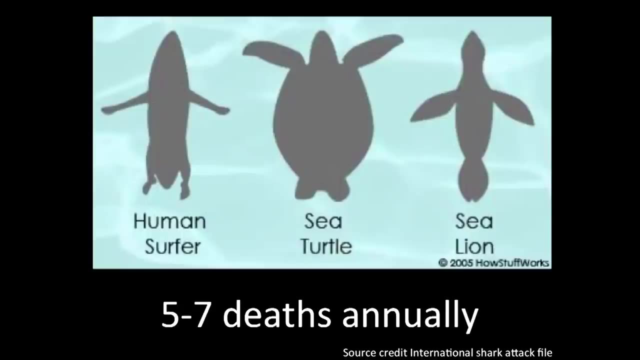 shaping and influencing them and making them stronger and better. Now, even though they are highly cognitive, cautious and taking multiple factors before they take action, it is true that on rare, rare, rare, much more rare occasions than we make mistakes, sharks do make mistakes. Unfortunately, someone does get bit Still. consider the millions of people that enter the water, the oceans, every single day, And the average number of fatalities is five to seven. Now I feel extremely lucky. I get to spend almost every single day diving with sharks. 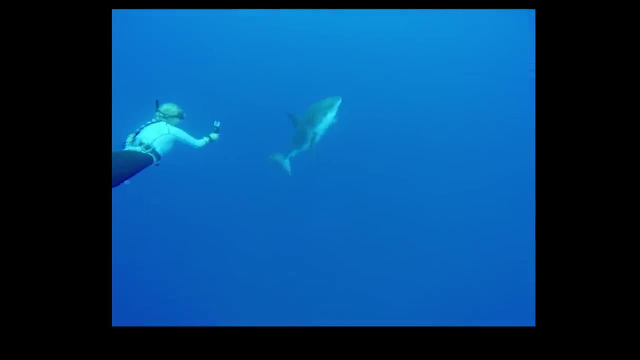 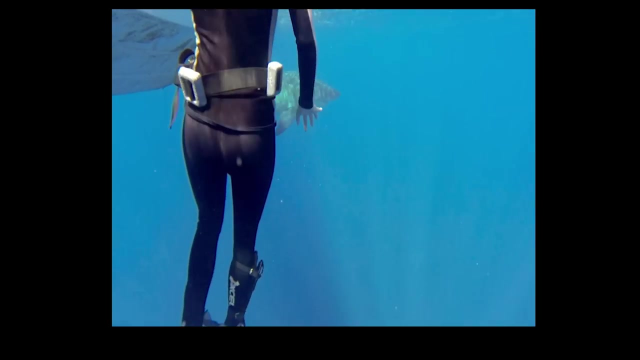 Over 30 different species around the world on a diversity of research programs and conservation campaigns. My work in marine biology focuses on ethology, which is animal behavior, and psychology and cognitive ecology, where I study the way the animals interact with one another and their environment. 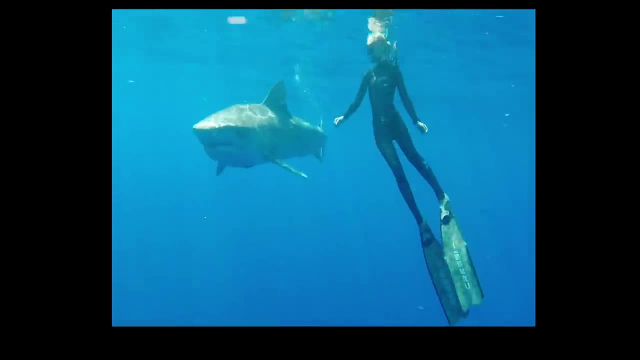 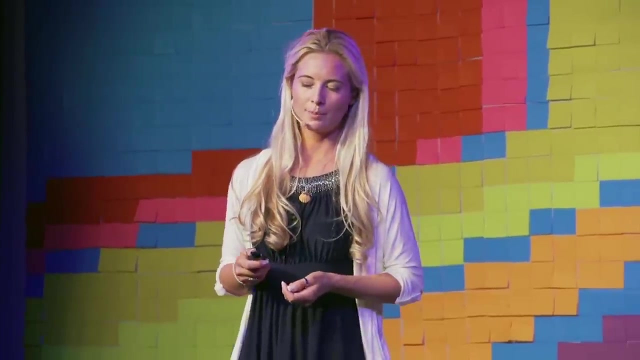 And I've come to observe and learn some of the most fascinating things that I wish I had more time to share with you tonight. But in my limited time with you, what I've come to appreciate what I feel is most important and urgent, 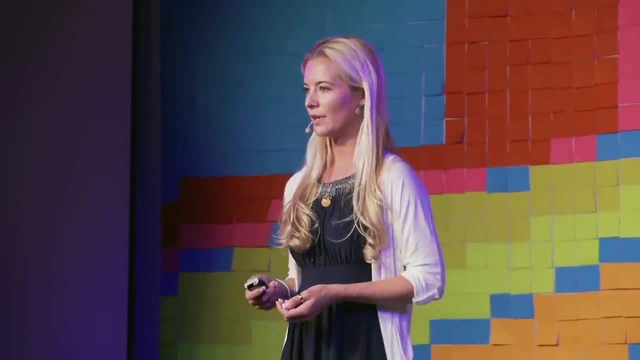 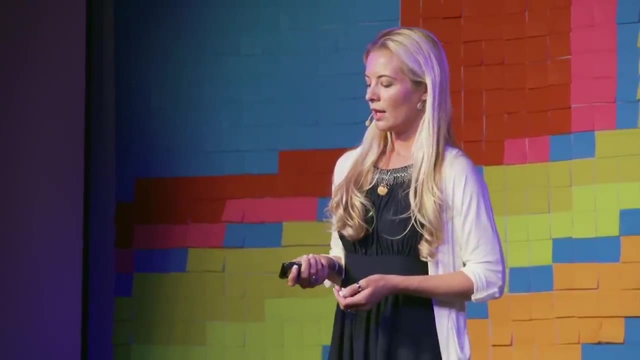 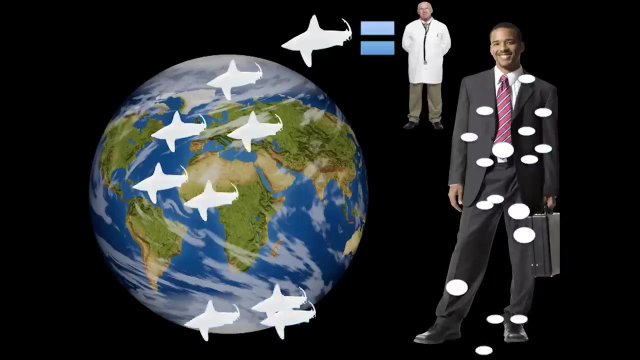 and if I could speak up for sharks, what I'd want to share with you is their very important role and work and how it affects all of our lives. Essentially, imagine sharks as the ocean's immune system, the white blood cells. They pick out the dead, dying, weak, sick, injured animals. 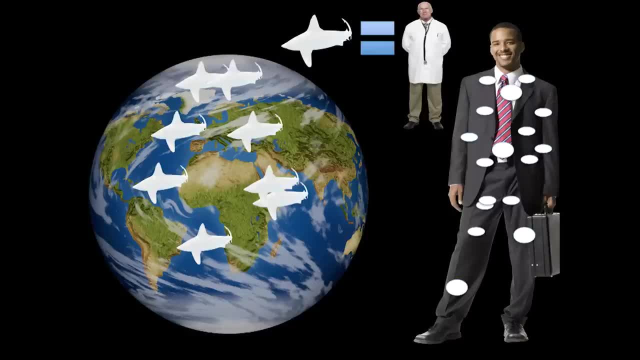 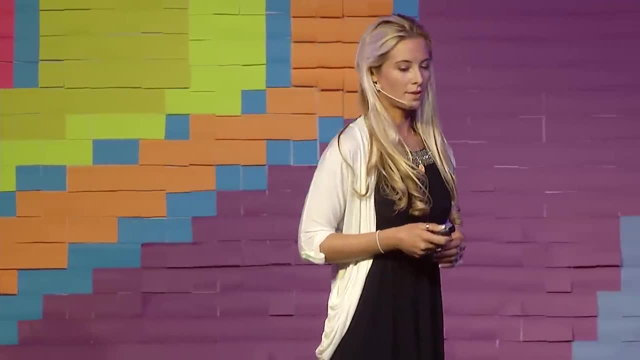 leaving only the healthiest to reproduce, keeping lower trophic levels and populations in balance. We all rely on our immune systems, and the scientific evidence for the importance of sharks is mounting. There are so many studies that show, one after the other. 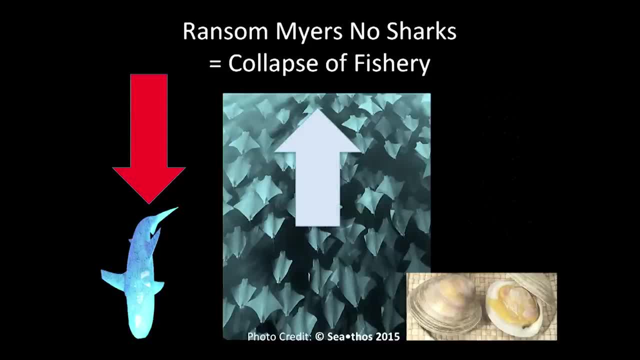 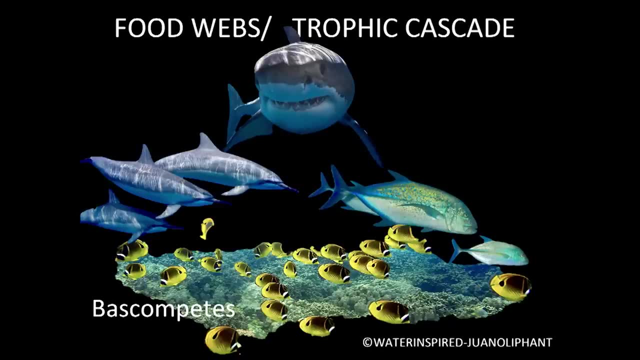 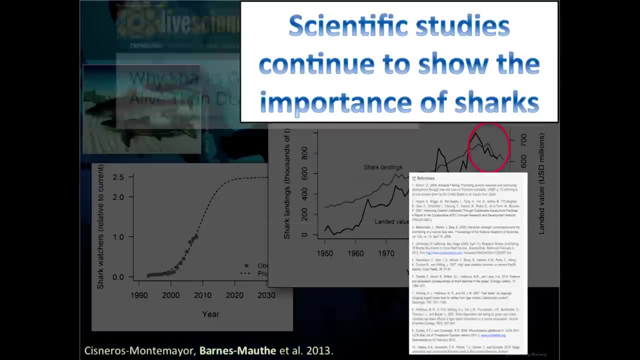 that the removal of sharks has environmental and economic negative impacts. Ransom and Meyer Bass Compete and effects all the way down to coral reef systems. The removal of sharks has been attributed with starvation Throughout the respective scientific community. there is no denying the importance of sharks. 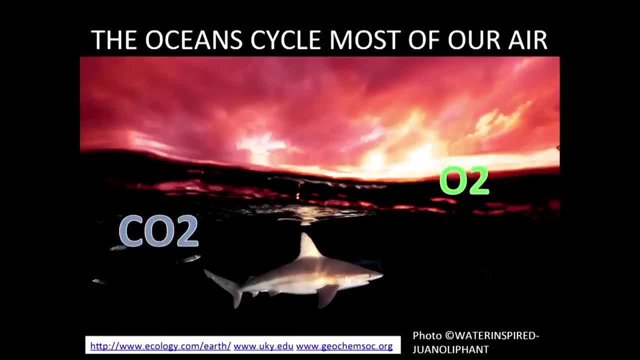 Their effects on our environments, our economies, even the air that we breathe- 70 to 80% of the air that we rely on to continue living- comes from our oceans. Either directly or indirectly, we all rely on the oceans. Billions rely on it for seafood. 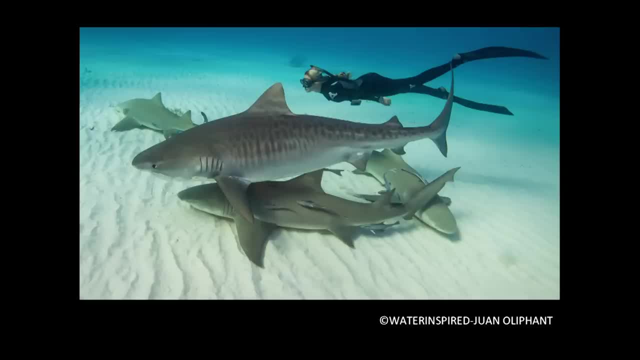 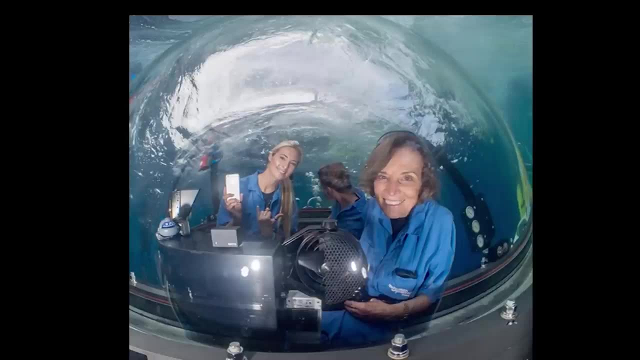 Over 200 million rely on it for dry food. Over 200 million rely on it for direct employment. Our lives, our futures, are interconnected- In the words of one of my human role models, the wonderful Dr Sylvia Earle- with every drop of water that you drink. 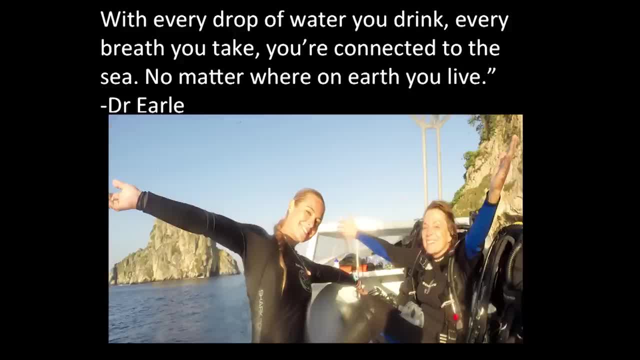 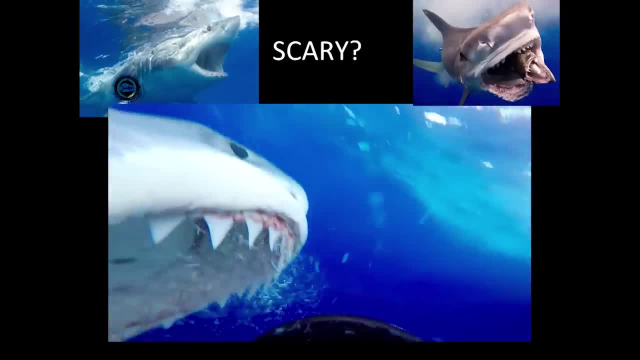 every breath that you take. you're connected to the sea, no matter where on the planet you live. So, but sharks are still scary right. So that's kind of the problem: Most people don't know many factual things about sharks. 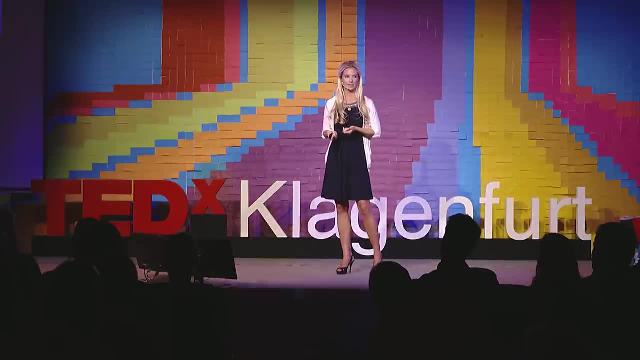 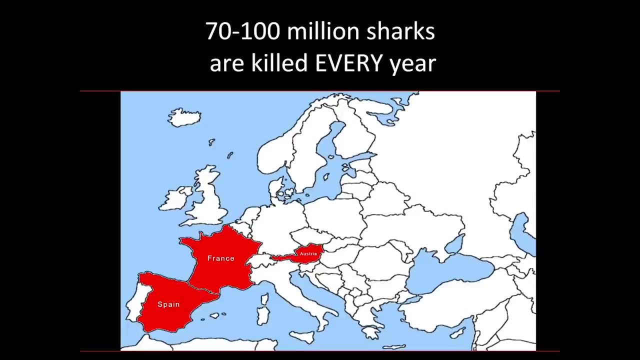 except that they have teeth. Most people don't know that sharks are actually being decimated globally at a rate of over 11,000 every single hour. That's more than three sharks every single second. That translates to 70 to 100 million sharks killing every year. 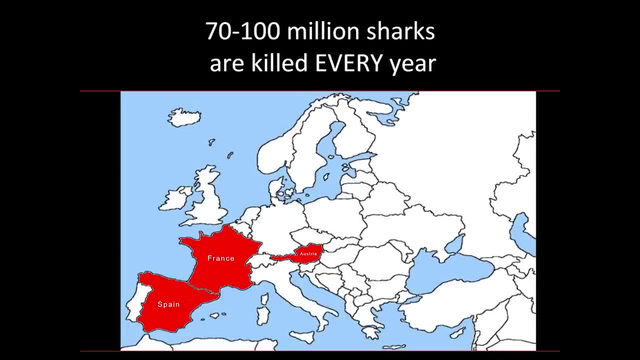 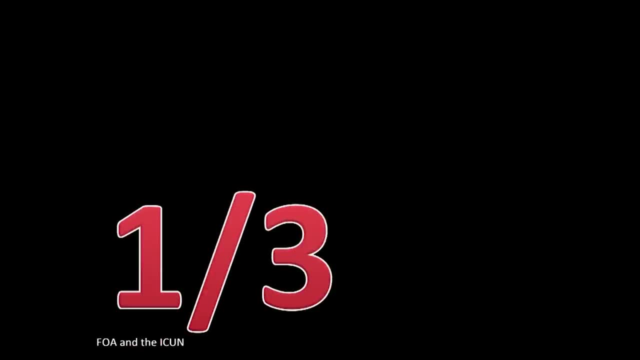 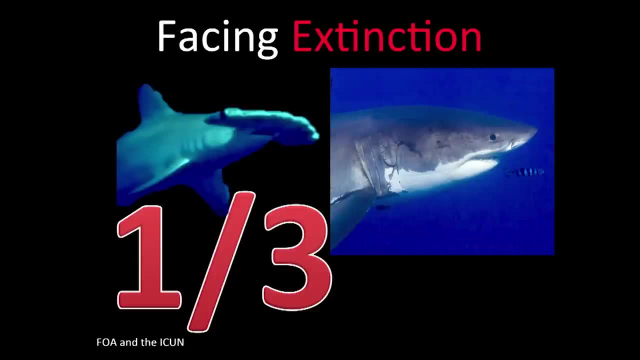 That's like killing everyone in Spain, Austria and France every single year. Now, according to fishing records, over 90% of sharks have been depleted. According to the International Convention for the Union of Nature or Conservation of Nature, over a third of all large sharks have been wiped out. 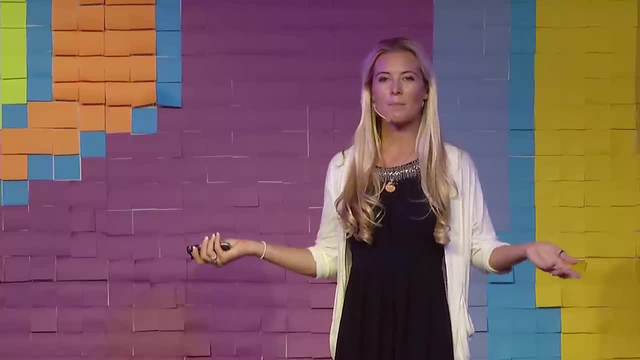 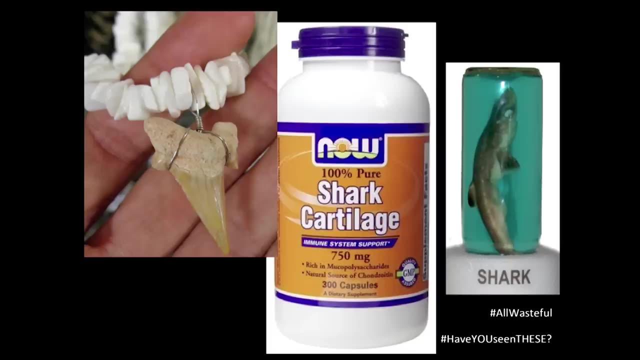 or are facing extinction or vulnerable to extinction. So why such a mass slaughter of such an important and keystone species? Well, some of it is due to silly things like souvenirs and pharmaceuticals. Some of it is due to men and their inferiority complexes, I'm guessing. 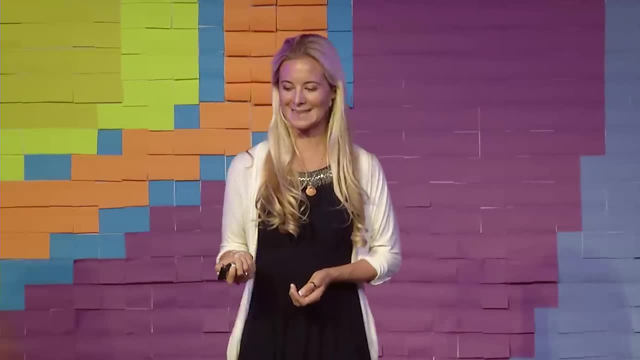 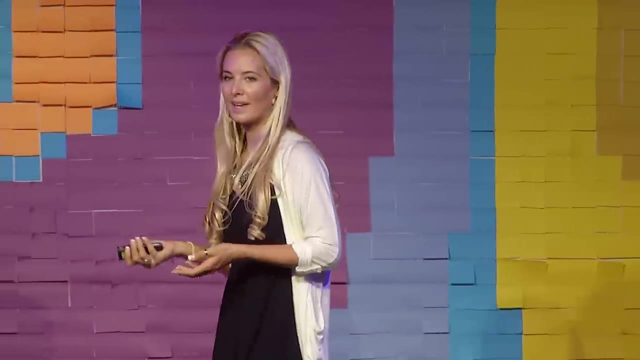 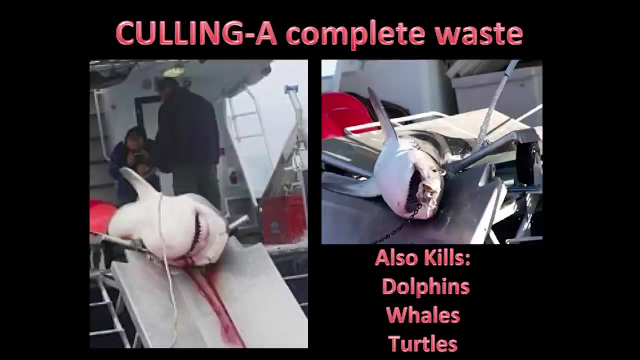 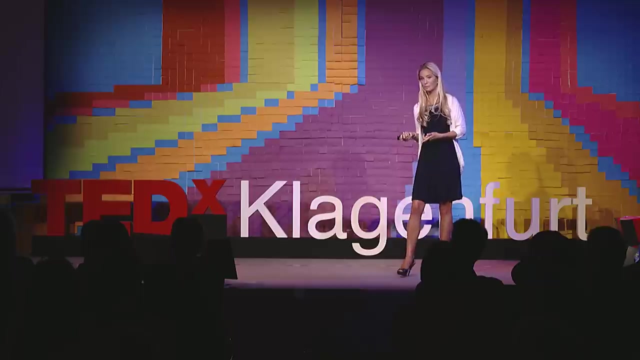 The shark. 80% of long-lining is bycatch and most of it is sharks Culling, which is probably the least intelligent reaction a country can have to an adverse shark-human interaction, basically like shooting yourself in the foot. from a behavioral standpoint, 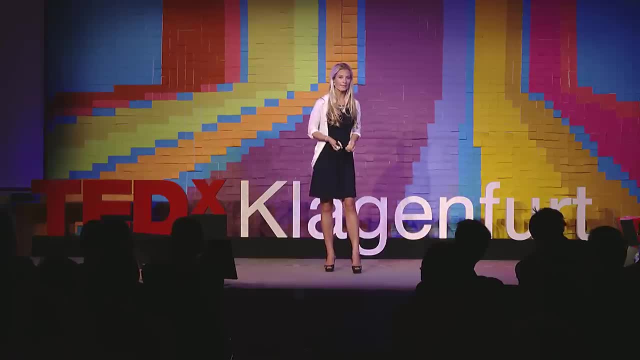 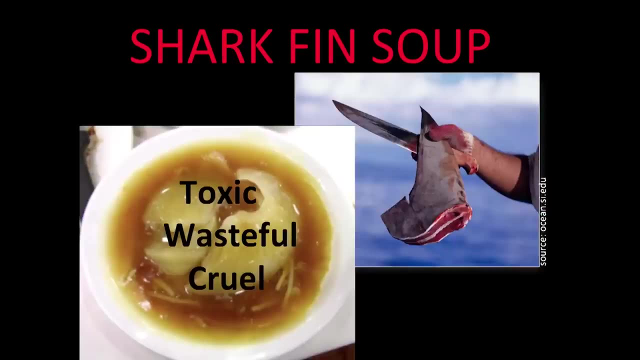 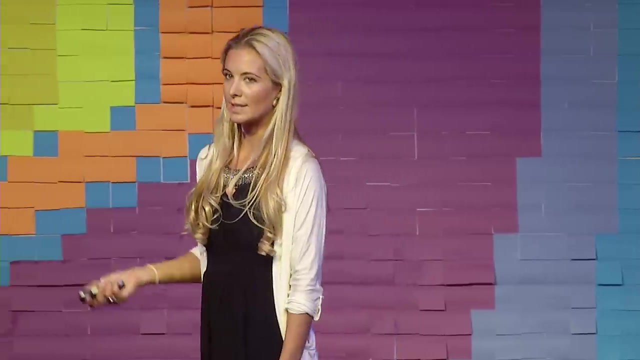 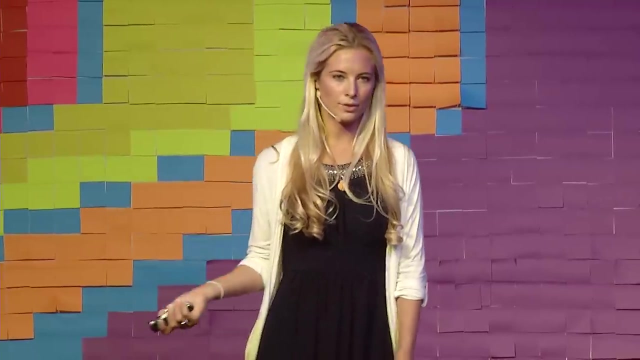 also a waste and indiscriminate killer. But the number one killer of sharks globally is a bowl of soup. Yes, we are trading the health and productivity of our ocean's reliant environment and economies for a bowl of soup. What's worse, it's not even nutritious. 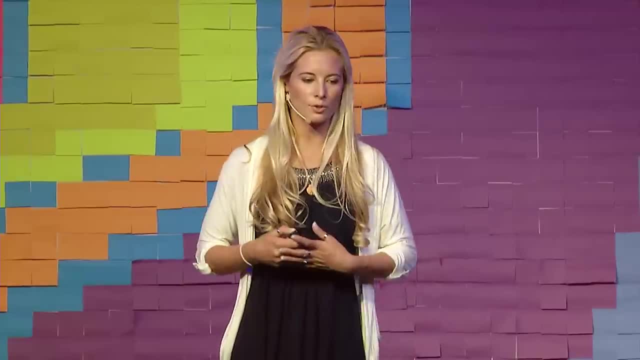 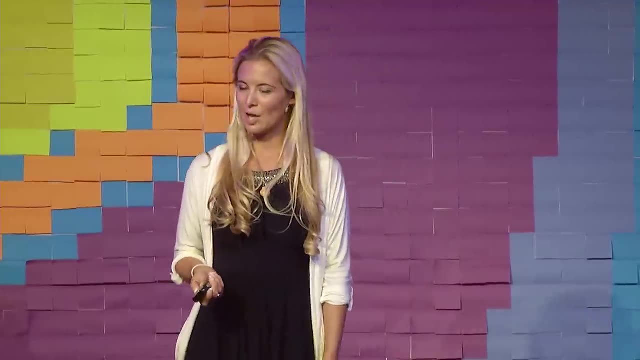 It's actually toxic. It's merely for the Chinese cultural belief that when they serve that soup it means that they're prestigious or important. But what is classy about catching a shark, hacking off its fins, oftentimes while it's still alive? 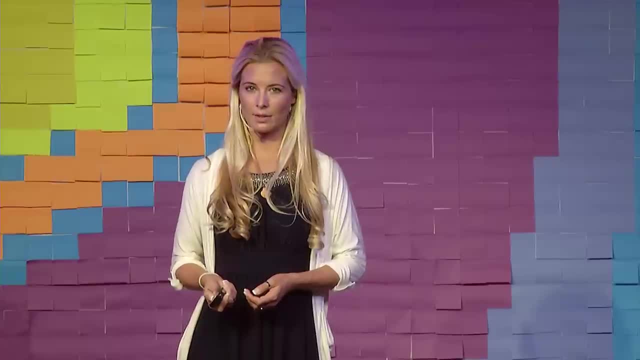 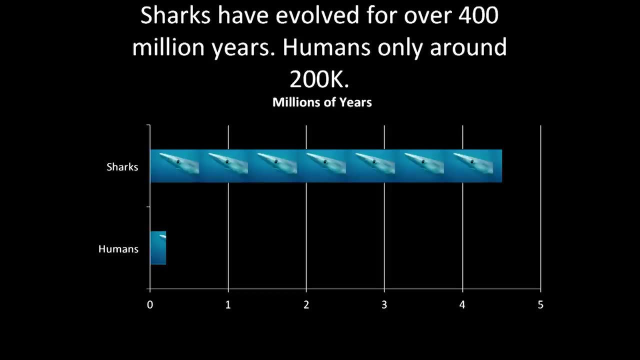 wasting 95% of the animal just to make yourself feel better about your social status. Consider: sharks have been evolving for over 400 million years, Humans 200,000. And their culturals far less. We can live without culture. 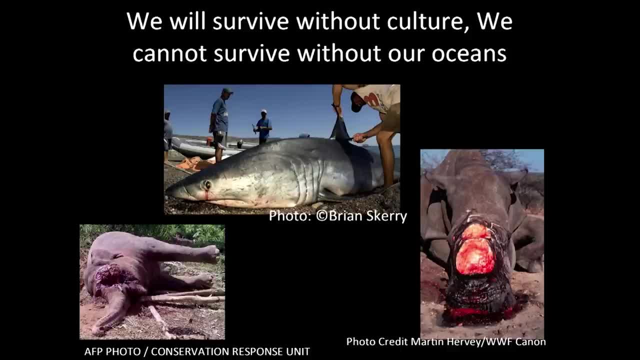 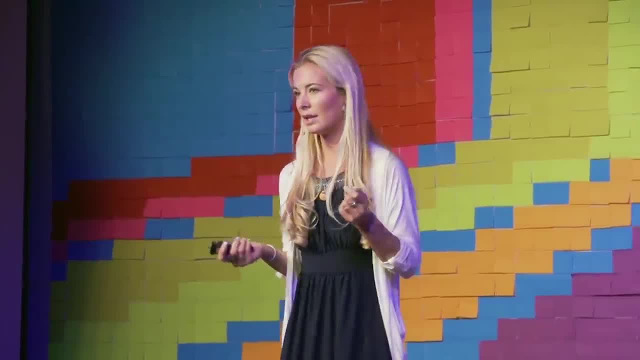 We cannot live without our oceans and our oceans cannot live without their immune systems. Like rhinos killed just for their horns and elephants killed just for their tusks, sharks are being killed, slaughtered, killed globally, just for their fins. Now, I love traveling the world. 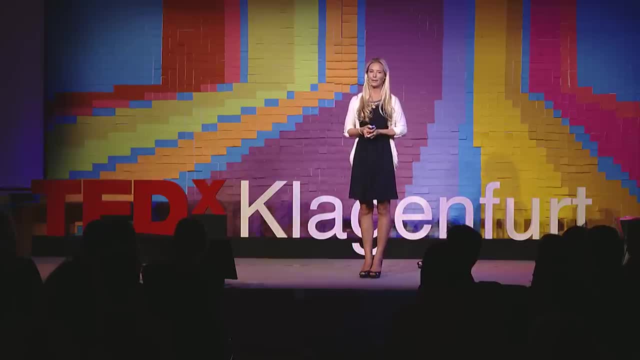 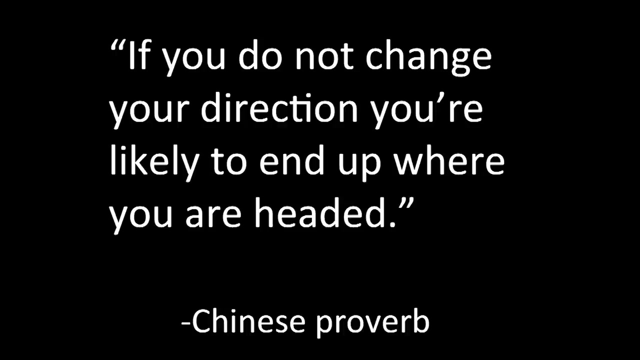 and experiencing the diversity of cultures, but there has to be a point when we reevaluate the relationship that we have with sharks and animals and look at how our cultures can adapt and evolve honorably. There's an ancient Chinese proverb that says that when you do not change your direction, 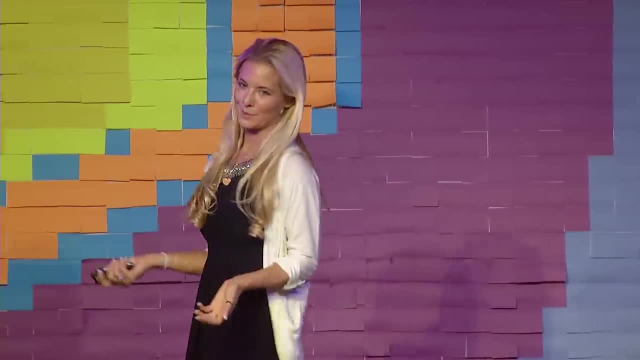 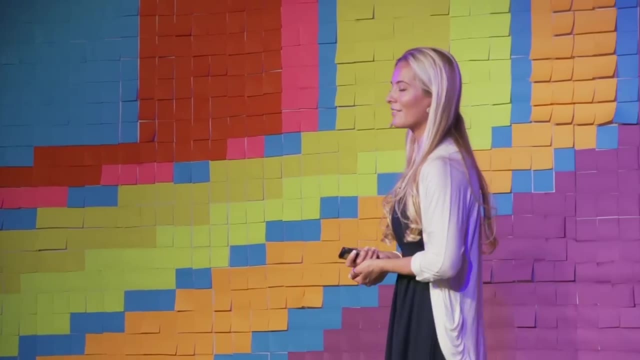 you may end up where you are heading. So what if we were to adopt this idea and change the way that we interact with sharks? What would that look like? Well, the great news is we already have concrete examples: places like Palau, Bahamas. 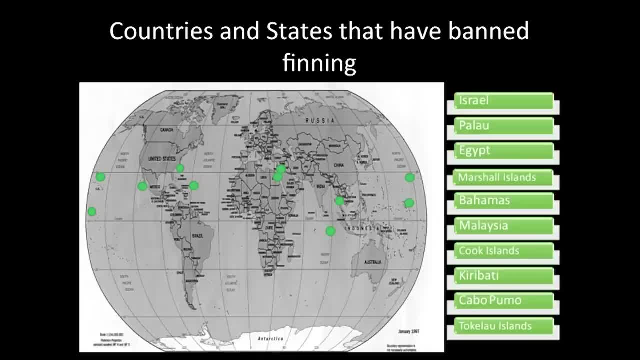 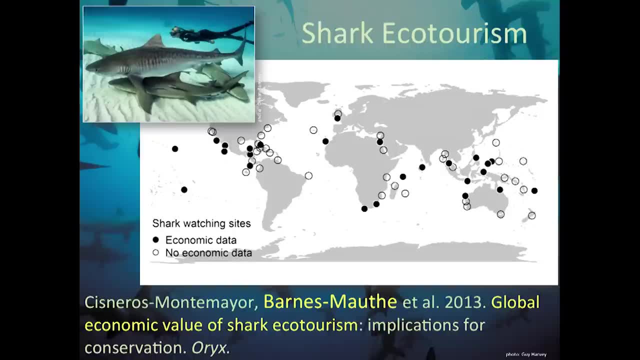 areas like Cabo Pumo and Palmyra, And in those areas, reef and fish stocks are thriving And ecotourism is bringing in over $314 million US to local economies, directly employing over 10,000 jobs. 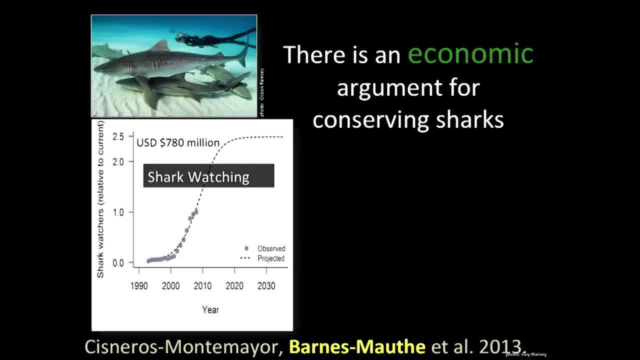 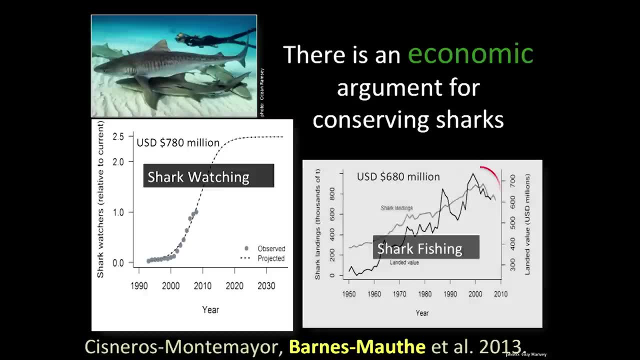 This study done by the University of British Columbia and Dr Michelle Barnes is actually showing that that number will increase more than double in less than 20 years to $780 million, Far outweighing the global fin trade. So, put at the most basic terms, 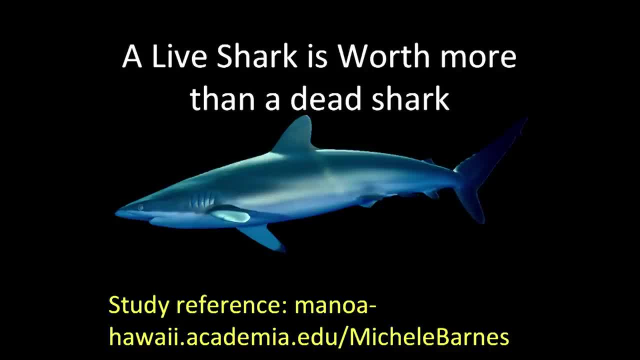 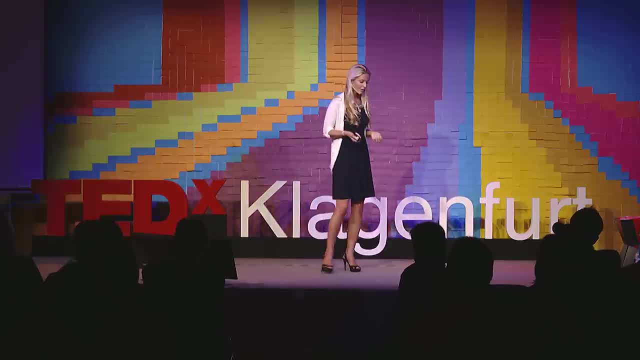 even on just the monetary level, which is usually what politicians care about, a live shark is worth more than a dead shark, And what's great is these shark ecotourism programs. they can support research, And so I was working out with Dr Mauricio Hoyos. 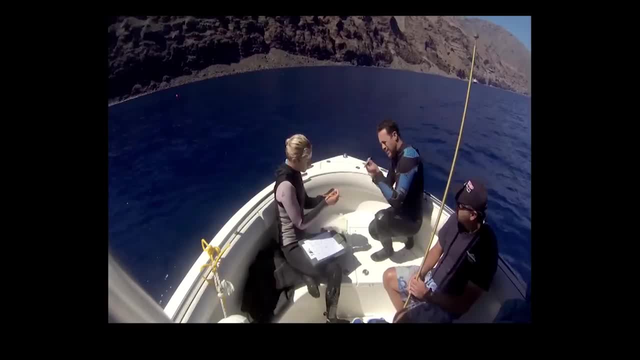 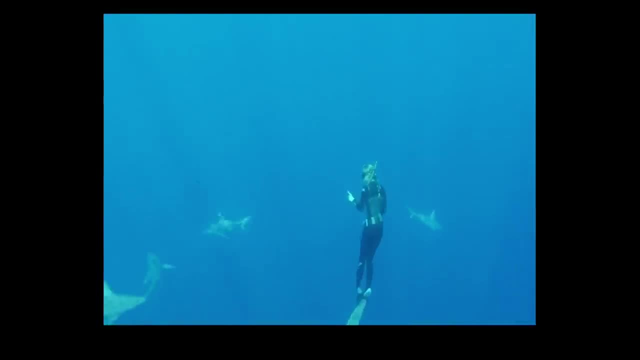 we were tagging, we were taking biopsies and I was wondering: is any of this conservation-based research gonna make a difference before these guys are just wiped out off the planet? And then one day, 20 meters underwater and I was doing a population count. 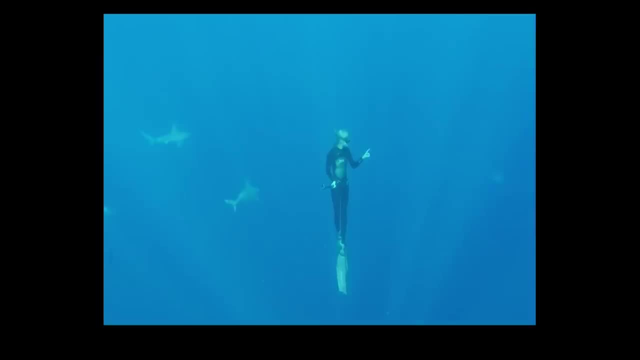 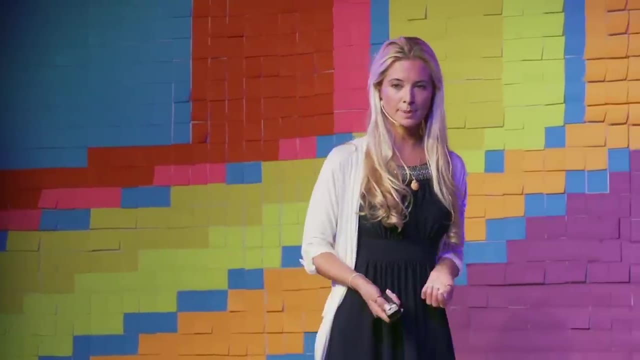 I was surrounded by all these beautiful sharks and I was realizing, by the time I gather, process and publish my studies, another three to six million sharks will be killed. So what's the point of studying something that's being eradicated at the rate that sharks are? 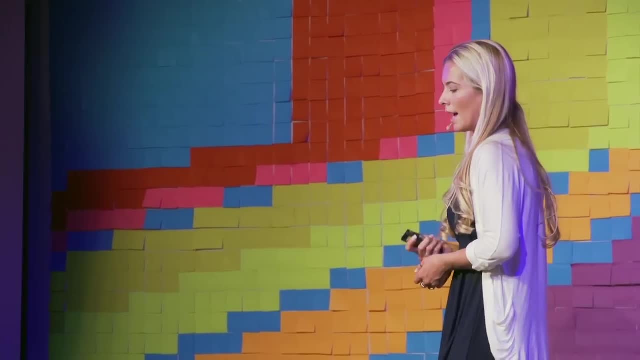 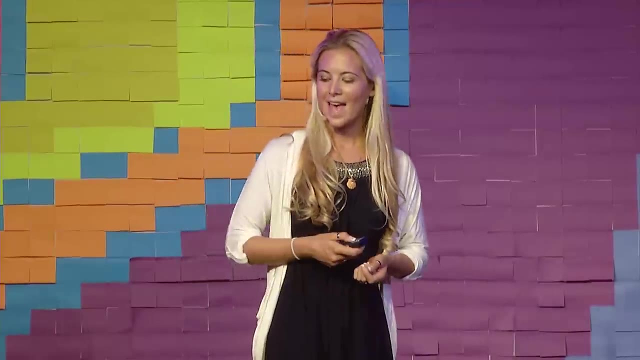 if you're not gonna do something about it. So I opened my research to the public. I developed a program where people could come to learn about sharks from a scientist, a scientific perspective, And I collaborated with Atwan Sharks, who's a well-known shark and marine photographer. 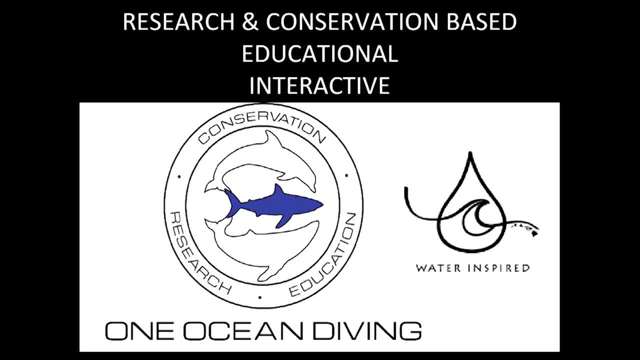 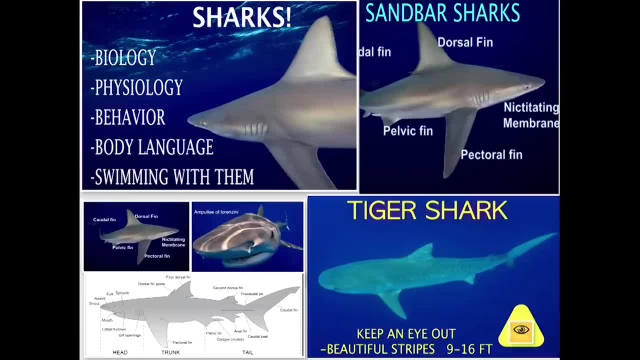 and shark specialist And we developed this program that's research and conservation-based and opened it to the public so that they could learn about the biology, physiology, behavior, body language, the safest way to interact with sharks, kinda answer all those questions that people. 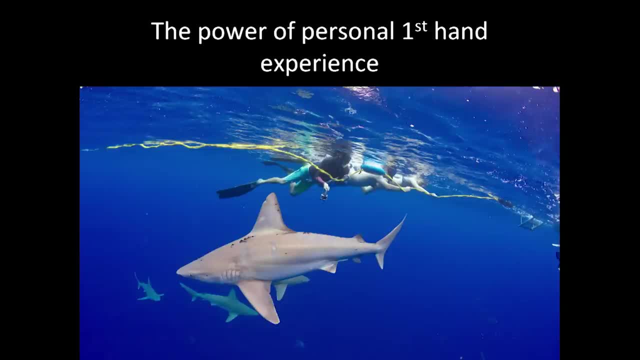 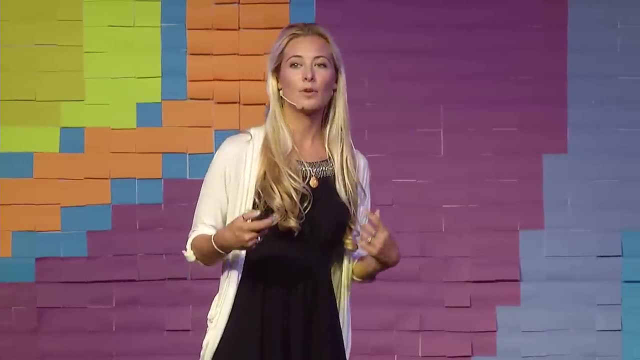 don't really know about sharks, And the cool thing is is people actually get to get in the water with us and see for themselves, eye to eye, face to face, what sharks really like. And it's such a successful program because people are able to speak up for sharks. 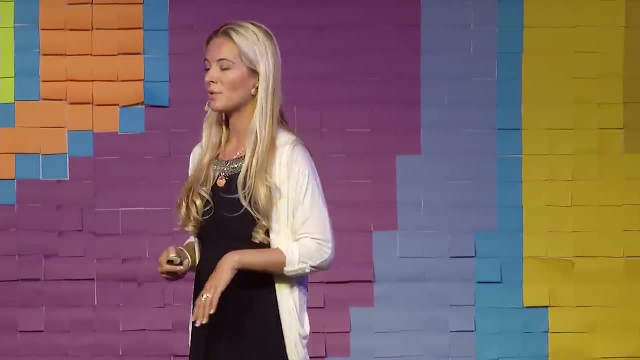 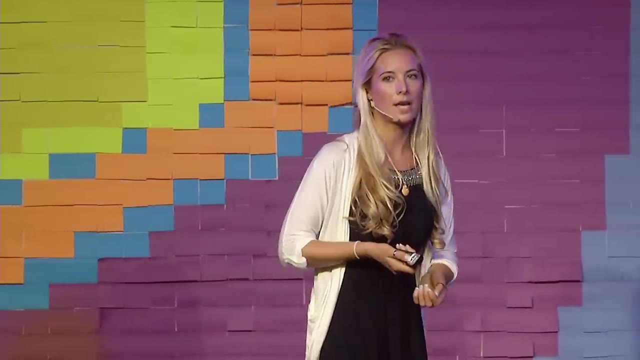 from a first-hand perspective, but also influence their networks and change people's minds. We are also able to fund educational outreach through this reef and beach cleanups, local conservation campaigns and international conservation campaigns, Like stopping the cull in Western Australia. 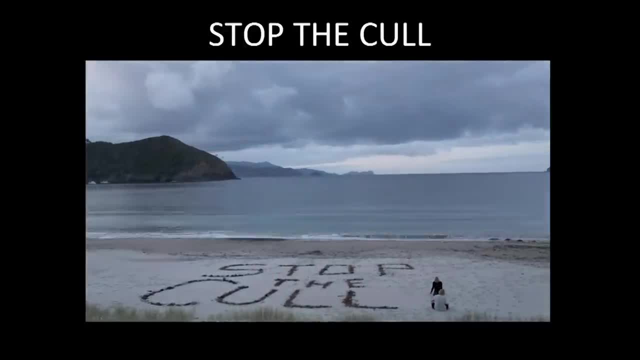 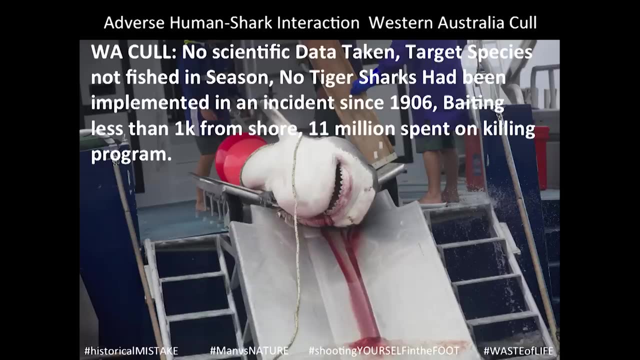 This is a story for another time that honestly, I'm kinda glad that I don't have time to share tonight because I would end up crying. But we were able to save one of the juvenile sharks. she was under three meters and she would have just died. 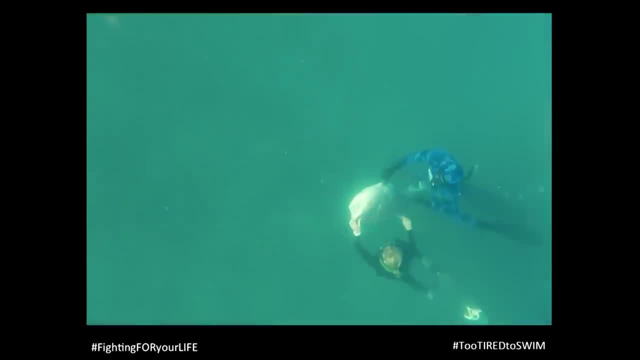 even though she was cattle tagged improperly. And you know, for 90 minutes I swam with her, looking her in the eye and trying to like kinda tell her it was gonna be okay, as blood was spewing out of her head. 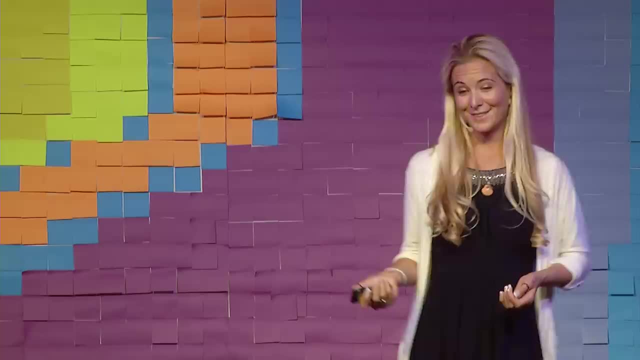 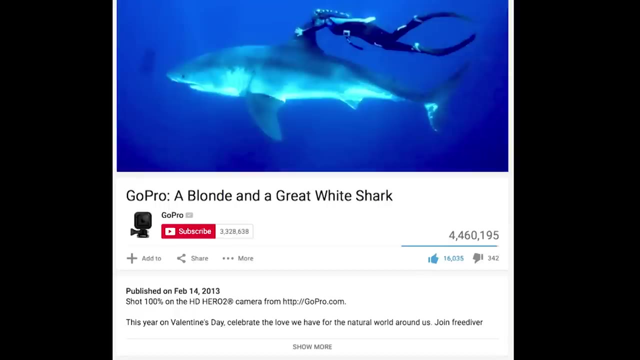 And kinda trying to tell myself that it was gonna be okay. and you know, after 90 minutes she swam off And it was that effort. This is another conservation campaign, a little bit more well-known. It reached over two million people in two days. 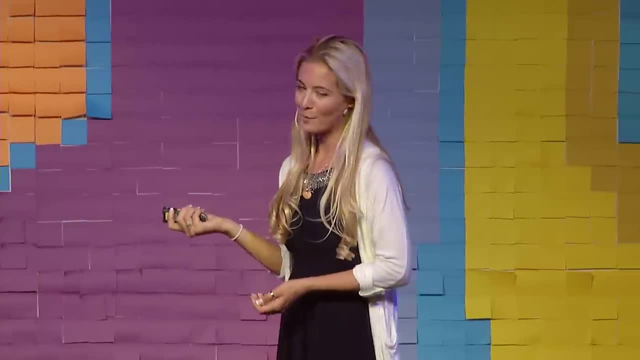 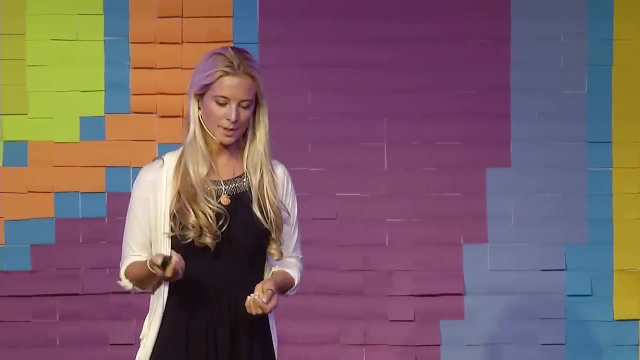 and featured 90,000 people. This is none other than the lovely role model, Bella, who is so great for her species, Great representative, And at the time when we released it, it was because there was a study that was put out. 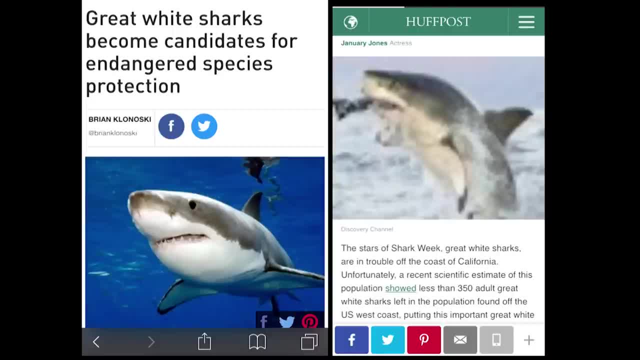 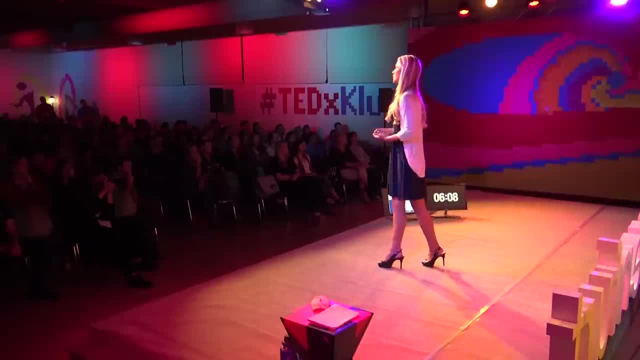 that showed that there were less than 350 great whites- And the area from California to Alaska, to Hawaii, to Mexico. that's an area that Juan Sharks and I grew up diving with sharks, with white sharks specifically. We knew a lot of these individuals. 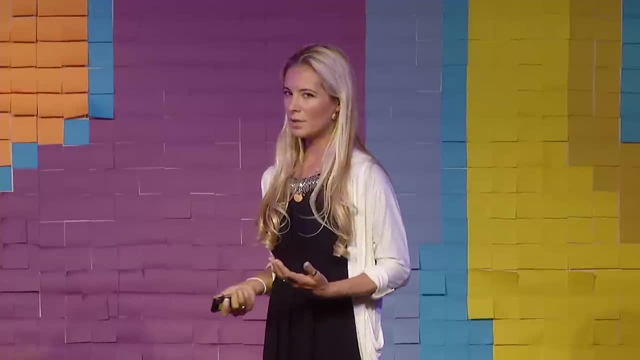 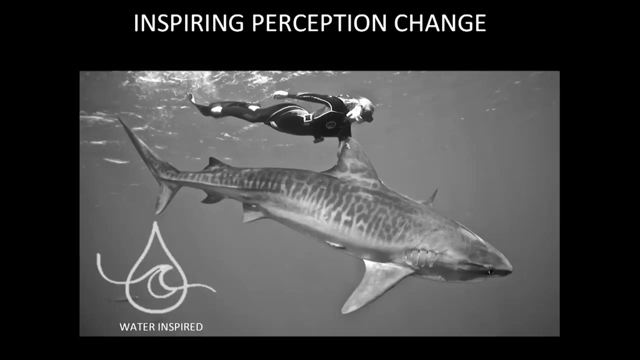 and had spent a lot of time with them, studying behavior and working with them. And so what do you do when you hear someone that you love that you care about being eradicated? You do something, And so we thought with Water Inspired. 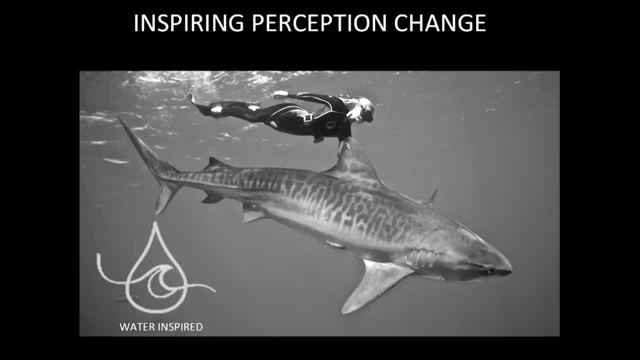 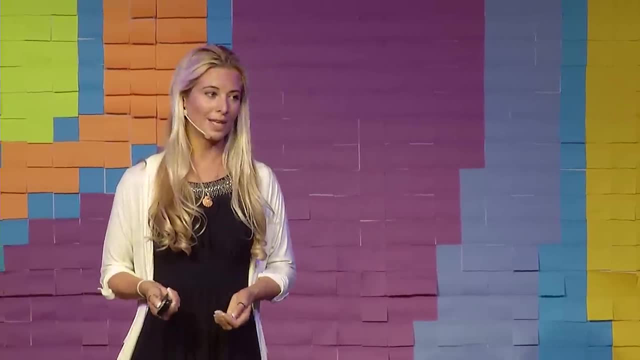 we try and use inspiring photography and videography to inspire people to care. So we needed people to give white sharks a second look, a second chance. They don't make the news very often and when they do, I'm sure you guys all know. 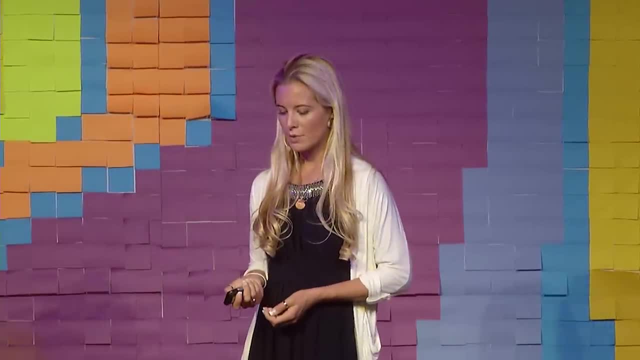 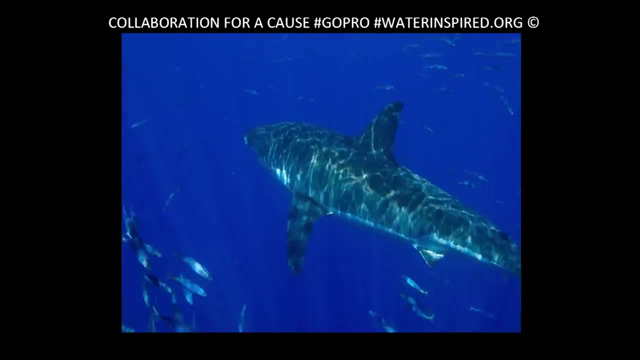 it's not usually a good press, So we were successful. We wanted to show the natural beauty of sharks, But most of the time when people see a beautiful image like this, they just think, oh, it's just on its way to eat the next person, right? 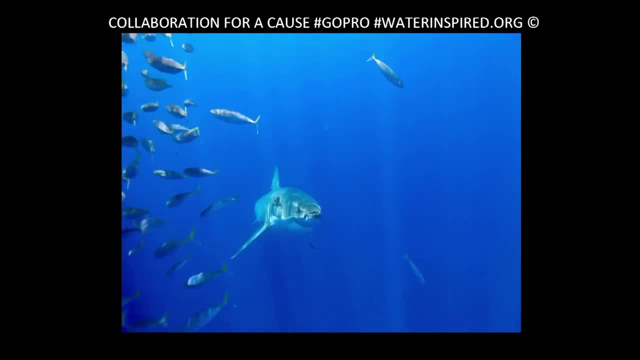 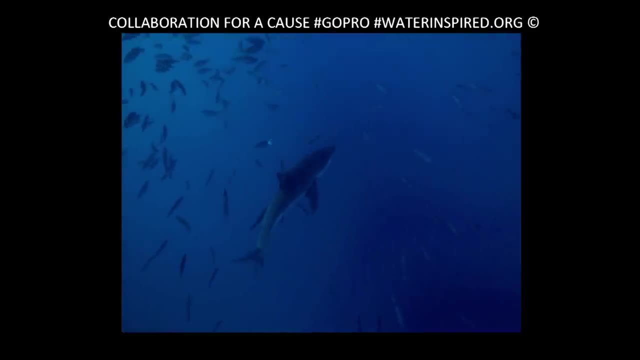 So we want to do the anti-jaws. The little blonde girl: she gets eaten in the fictitious movie, right? So what's it like in reality? Well, I've been working with them for a long time, right? We dive to get receivers and other things like that. 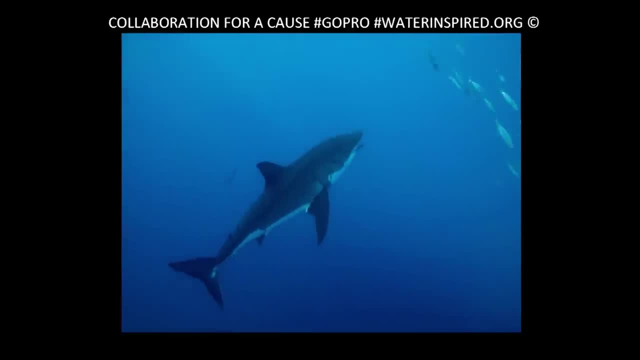 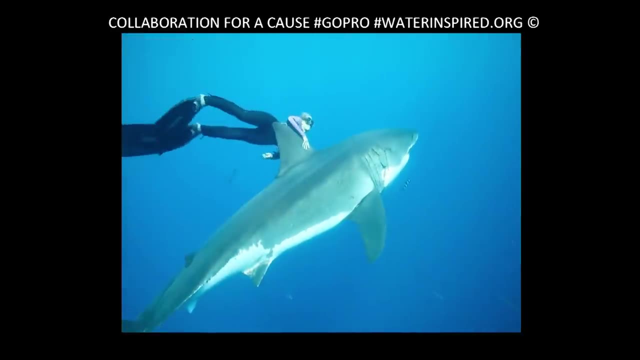 So I wanted to show a connection. I wanted people to be able to connect and see another side of these animals and realize that we can coexist. But in order to coexist they have to exist, And there's so much more to these animals. 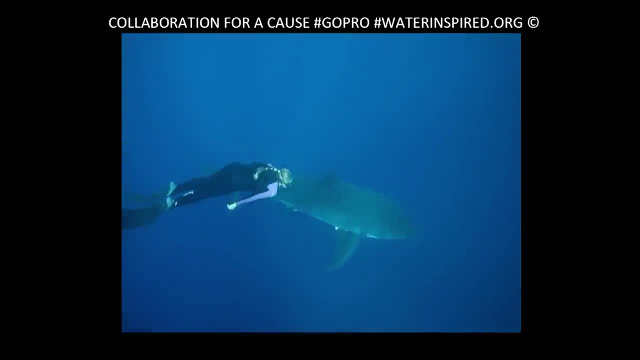 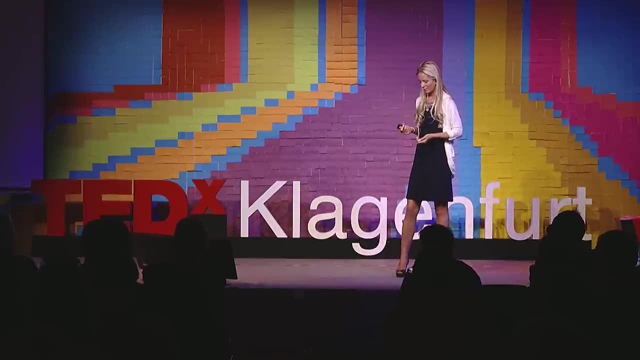 than meets the eye, And so when you take the time to get to know somebody you know, you can understand that maybe there's more to them, And so I wanted to share that with the world, And I have to give the disclaimer. 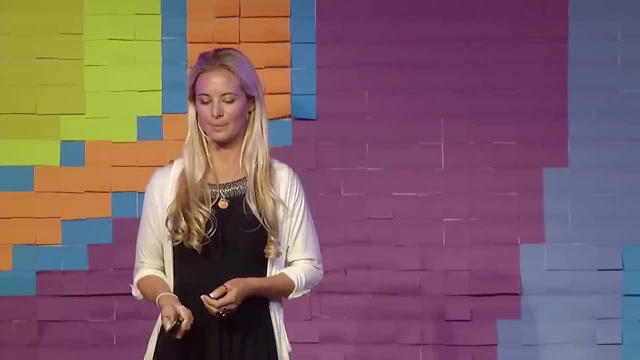 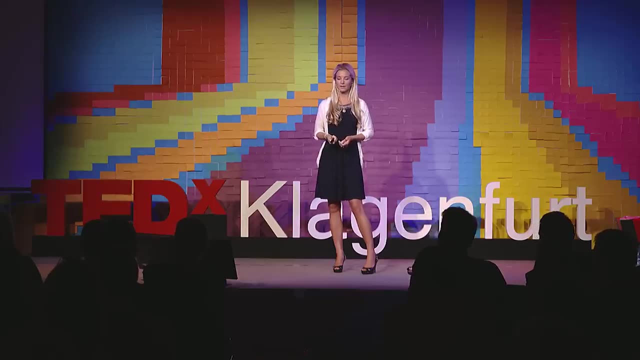 I mean so many things that I would love to share with you guys, But I do have to give the disclaimer that they deserve a lot of respect, not fear, But they are apex predators. They do have a role And we need them for that role. 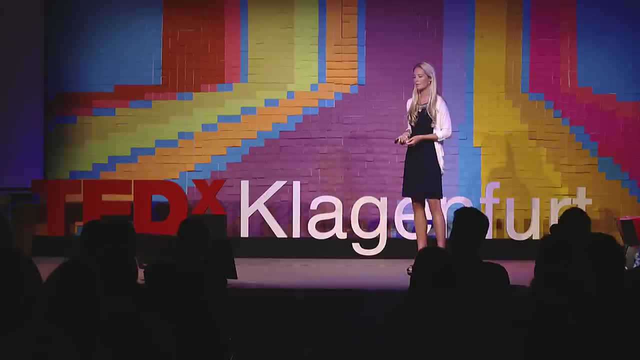 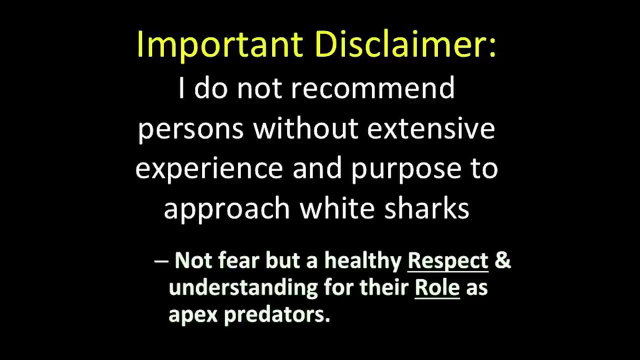 It's very important. I mean, I could cite study after study after study showing the importance of that. You know, if I wanted to go out into the African savannah and pet a lion, you know what I would do: I would call up the Lion Whisperer. 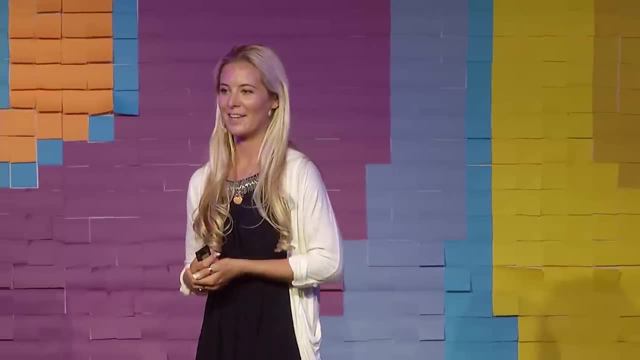 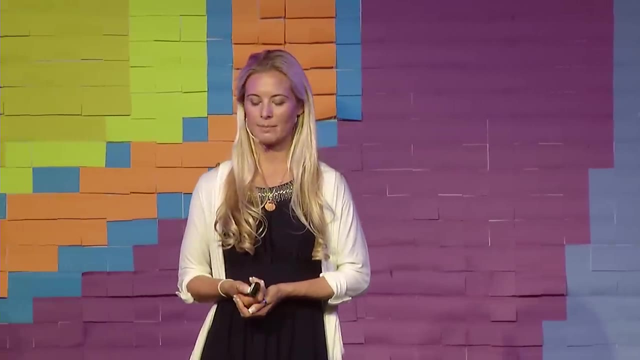 and I'd go hang out with him And I'd learn and I'd study from him out of respect for the animal because of its reputation. So, while I understand that, especially the way that they're portrayed in the media, that people are afraid of them, 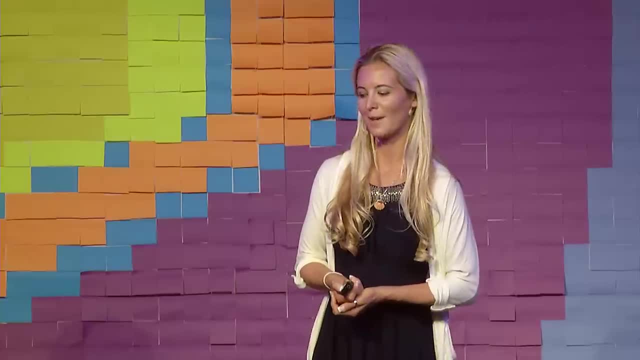 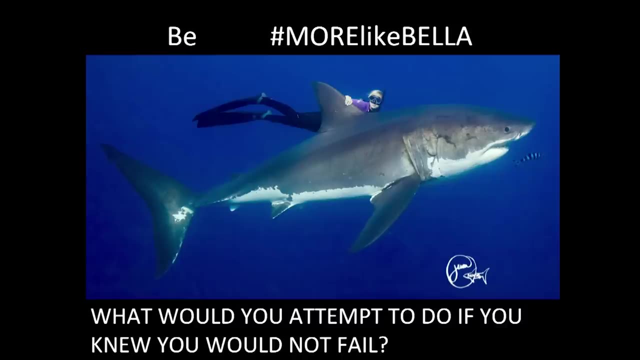 you shouldn't be afraid of them. You should just respect them. They're beautiful animals. There's so much more to them. So if there's one thing that Bella's taught me, it's that, like Bella, we can all positively change and influence our environments for the better. 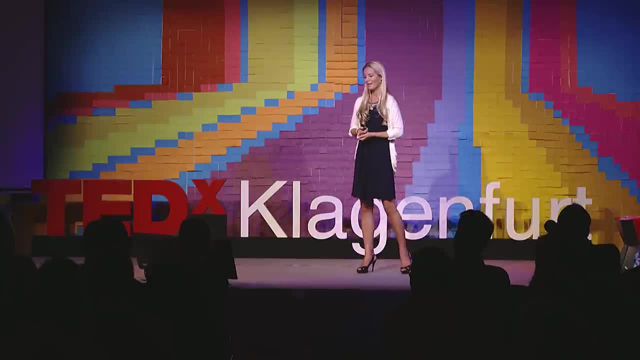 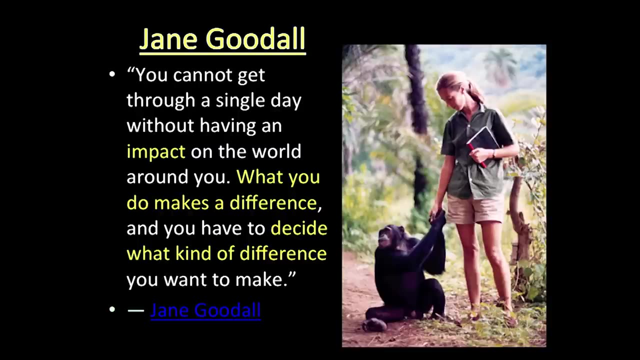 All we need to do is take action. In the words of Jane Goodall, every day we make an impact. It's up to us what kind of an impact we want that to be. Now. this was just one successful collaborative program that we collaborated with GoPro on. 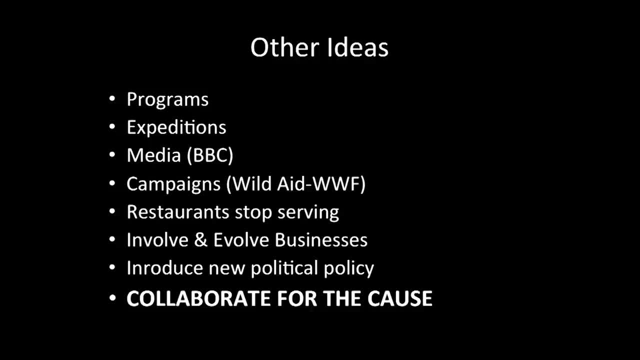 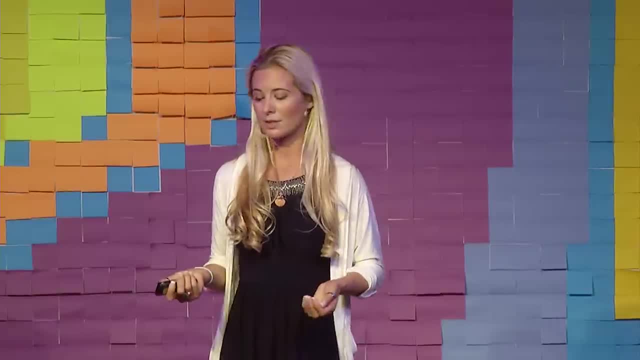 and they were very true to the message and released a beautiful piece. But there's so many other things we could do, So many other media pieces we could do, Even just writing to a restaurant and asking them not to serve shark fin soup. New campaigns, political policy. 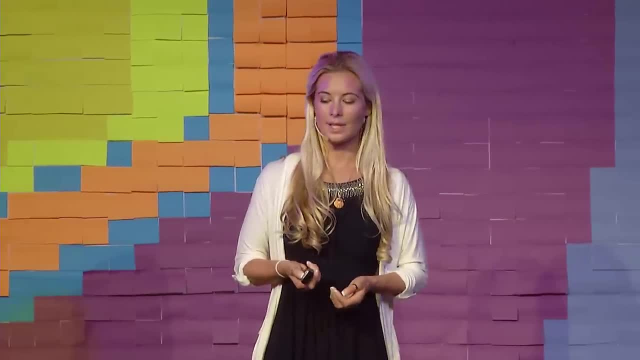 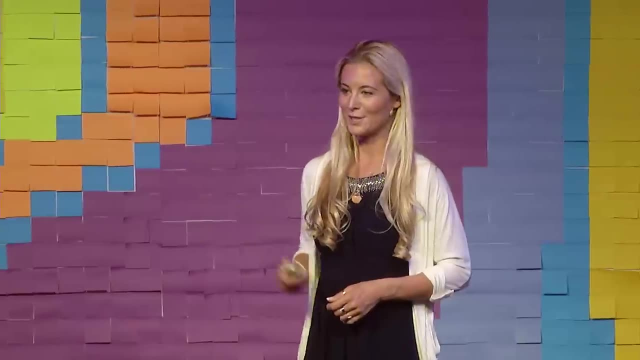 the ideas are endless. What it really comes down to is, yeah, knowledge is powerful, but it's nothing without action. I love Nike. I get up every morning and go running. It's like, just do it. You may not feel like it. 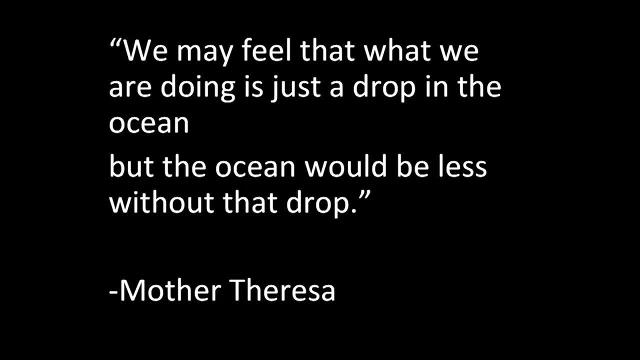 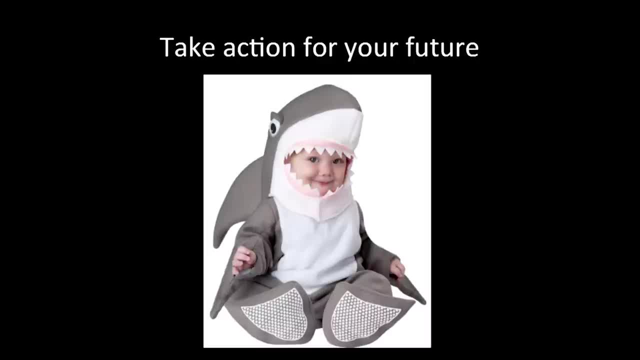 but you know what: Any effort's better than no effort at all. We may feel like what we are doing is just a drop in the ocean, but the ocean would be less without that drop. So I want to ask you guys tonight to take action for your future. 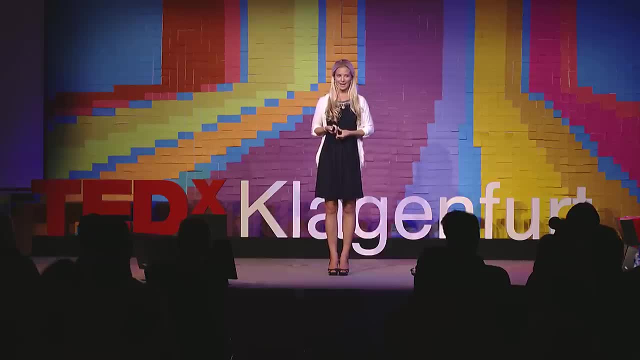 Sharks and the oceans affect us all And I'd like to see a raise of hands for all those that are willing to take a small, small action for a better future. If you guys can raise your hands, if you're willing to take the action. 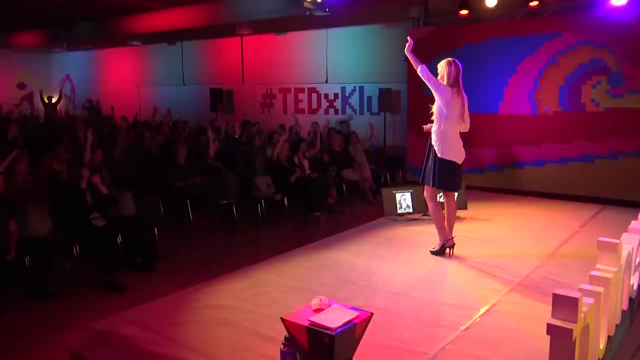 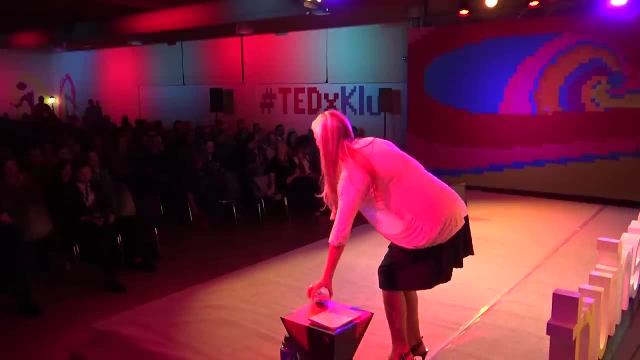 I love to see all those hands. Okay, now I'm going to call you out on it. I want you guys to use that hand and grab your phones. I'm going to do it with you. Yeah, grab your phones. I know it's usually rude to grab your phone. 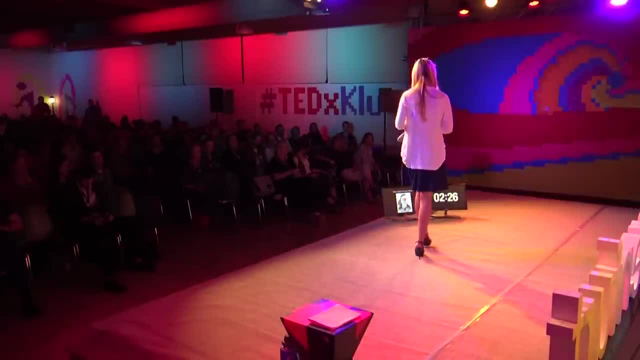 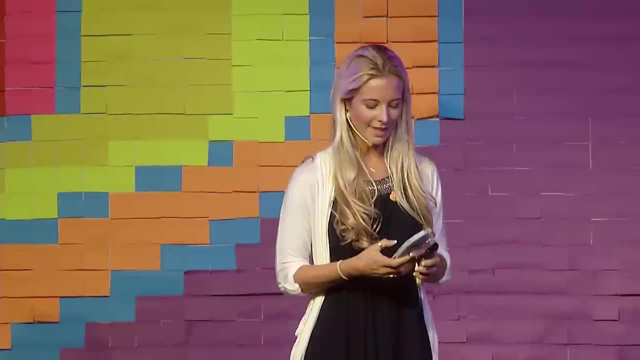 during a presentation. but this is okay, You guys are going to help me. This is really good. This is actually. this is good. This is your call to action. Let's do it. So I want you guys to grab your phone. 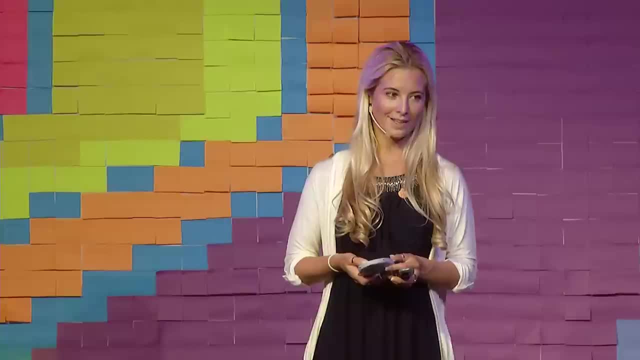 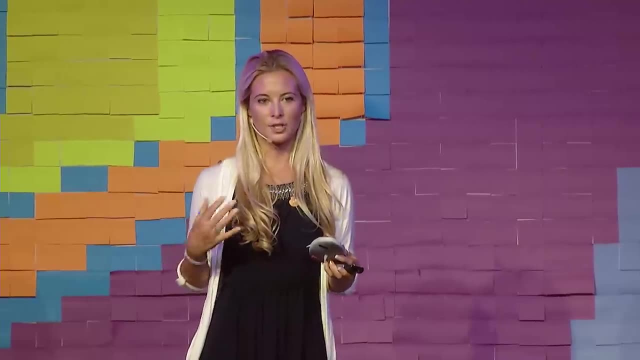 And we're going to spread great ideas globally. I want you guys to tweet Facebook, Instagram something, Spread an idea, Share a fact about a shark, And I'm going to do it with you because it's actually really fun. So, even though you guys are kind of dark right now, 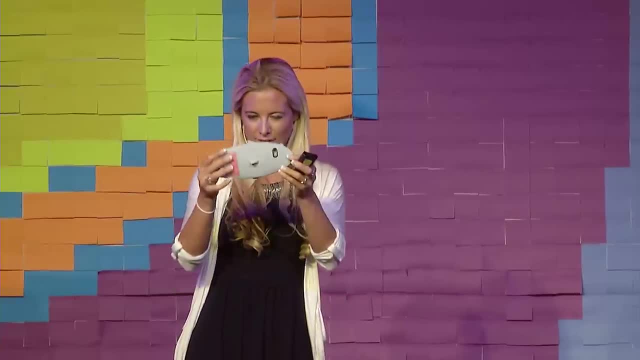 Okay, ready, Smile, Okay. So don't get distracted with the missed call or text. This is only going to take a minute and I'm off the stage. so, All right, let's do this together, because we're going to make a difference. 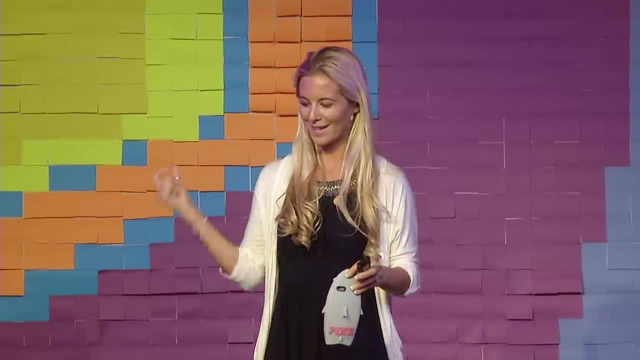 a measurable impact for sharks, So I'm going to Instagram. This is what the world looks like now. anyways, right, We all just walk around on our phones. I think I saw that on a talker, So I'm going to go to Instagram. 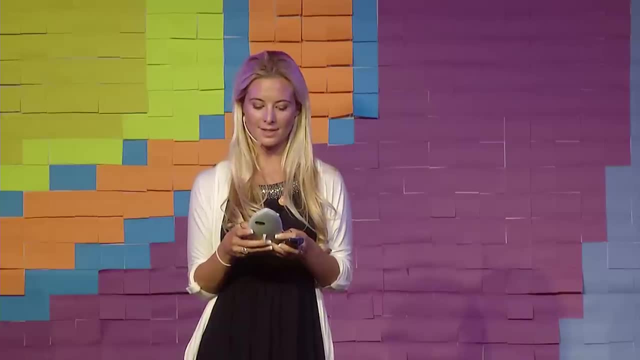 This is what the world looks like now. anyways, right, We all just walk around on our phones. I think I saw that on a talker, So I'm going to Instagram. This is what the world looks like now. anyways, right, We all just walk around on our phones. 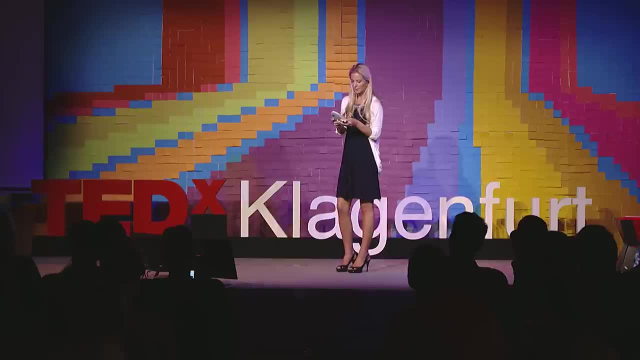 I think I saw that on a talker earlier. This is all good, Okay next. So I'm going to use a hashtag. It's a shark, help save sharks. It's a shark, help save sharks. Okay, Help save Bella. 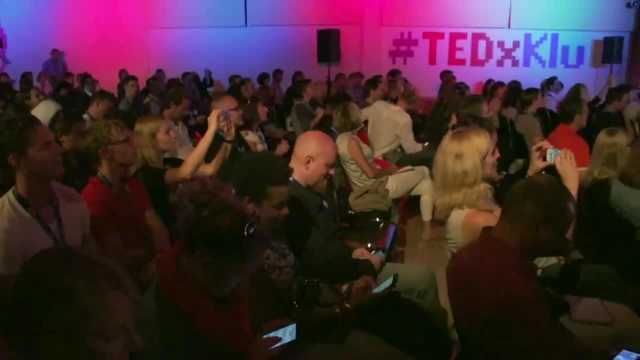 Here at the amazing group at TEDx Conference in Europe, helping spread great ideas and ways we can help save sharks in our future. Sharks are important, redefining the relationships we have with sharks and stronger relationships. Sharks are the most important to the science community. 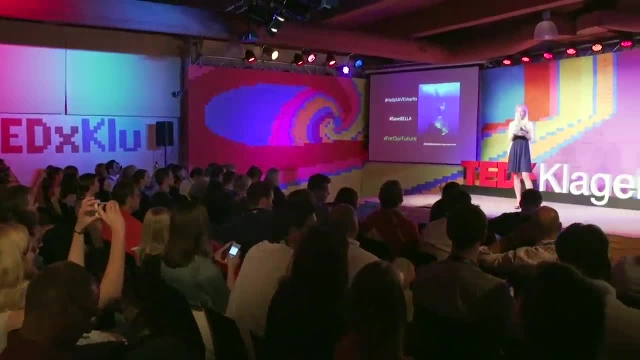 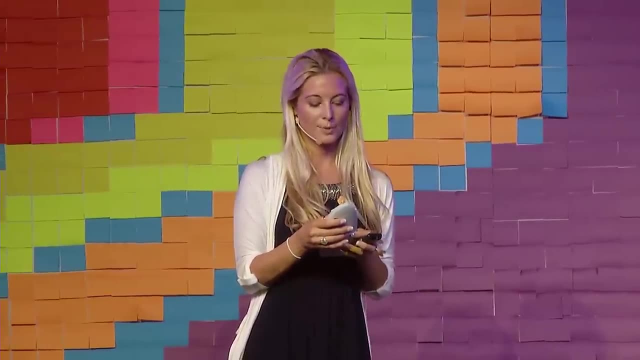 and the society. Sharks are the most important to the science community. Sharks are the most important to the science community. Sharks are the most important. are important redefining the relationships we have with sharks. shark conservation: help save sharks. no shark fin soup. Ted save sharks. Ted talks on sharks. 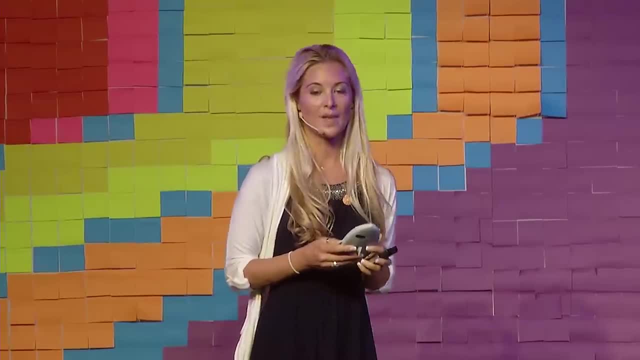 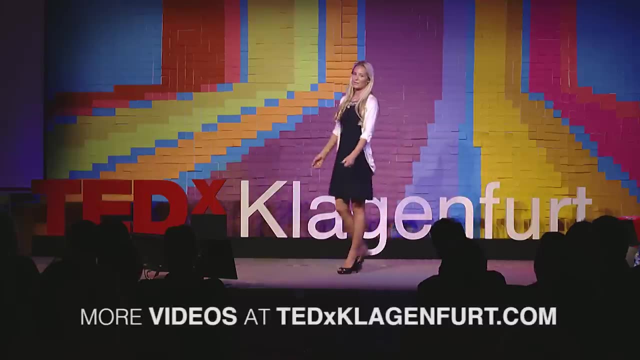 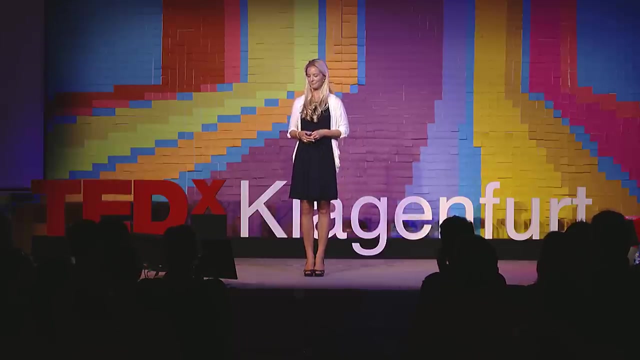 OK, And I will share that Awesome And this is the best part- I get to thank you all for being a part of the forest that redefines the relationship we have with sharks for a better future. Thank you guys, Thank you. 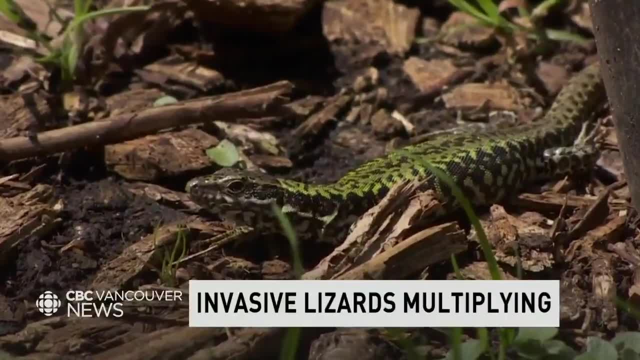 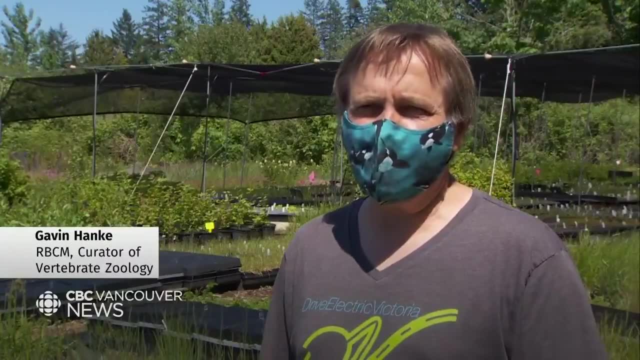 Wall lizards. the adults generally have some green colour to them and the scales on the back are really tiny- about the diameter of a sewing pin. Hi, I'm Gavin Hanke at the Royal BC Museum and here on Vancouver Island we have a serious lizard problem, The first wall lizards- only a few- were released here in 1967 in Saanich, just south of Brentwood Bay, and then in 1970 another 12 or so were released in the same area, and the problem we have now just stemmed from those few lizards that were released.